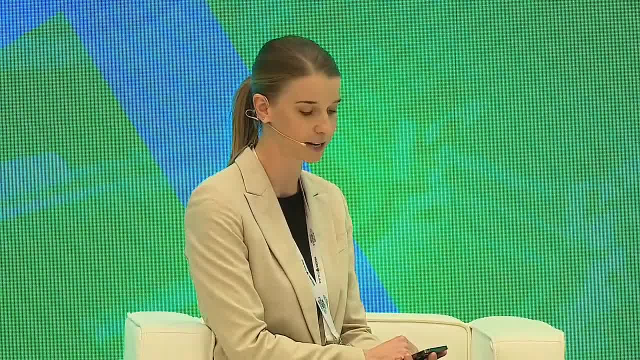 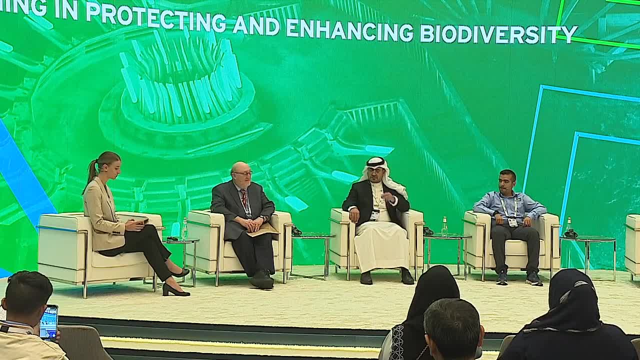 panel here To my left. it's Dr Murray Hitzman, director of the Science Foundation Ireland Research Center in Applied Geosciences, ICRAG. Mr Khalid Al-Sharif, vice president of strategy and planning at Marden, the largest multi-component mining organization in the world. 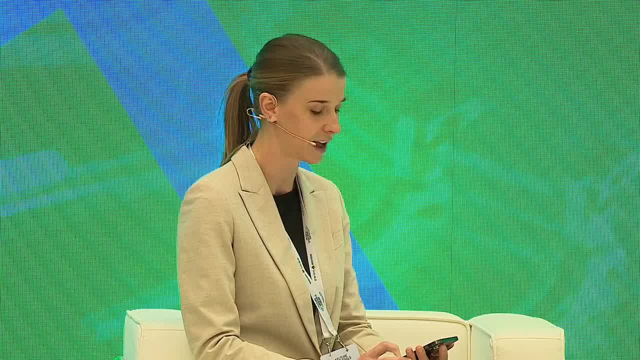 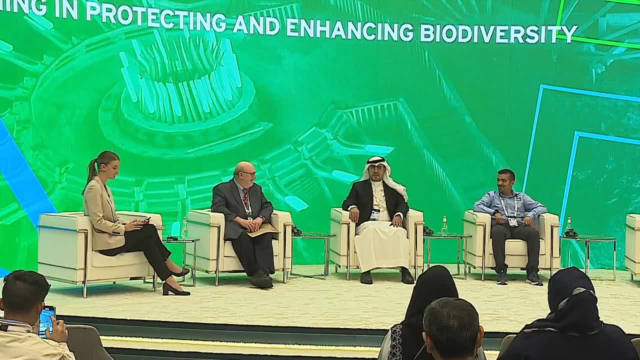 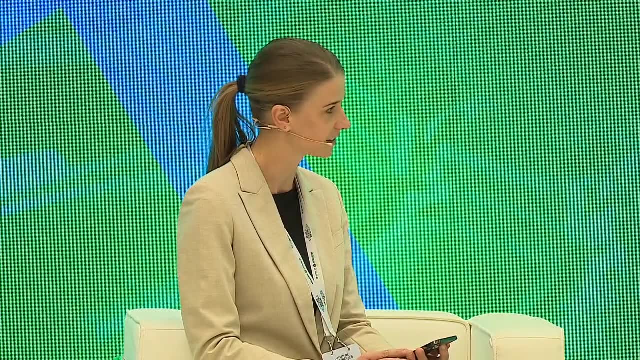 He's also the CEO of the commodity mining and metals company in the Middle East And, last but not least, Mr Hassan Al Ghani, operation development manager at Saudi Comedat, one of the leading contractors for open pit mining in the kingdom of Saudi Arabia. Murray, let's dive right in. 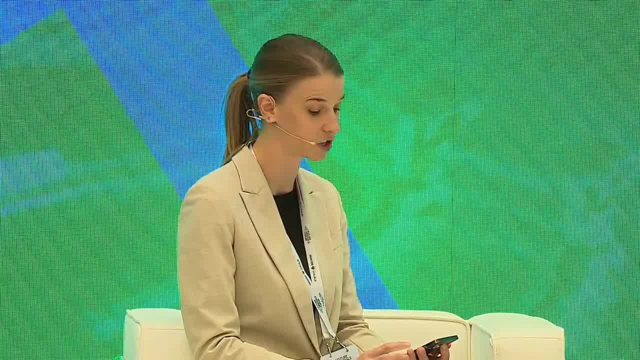 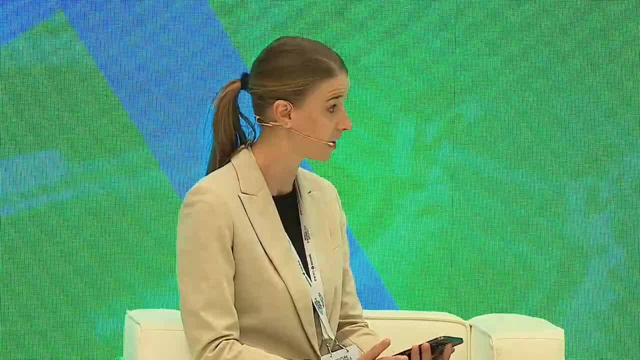 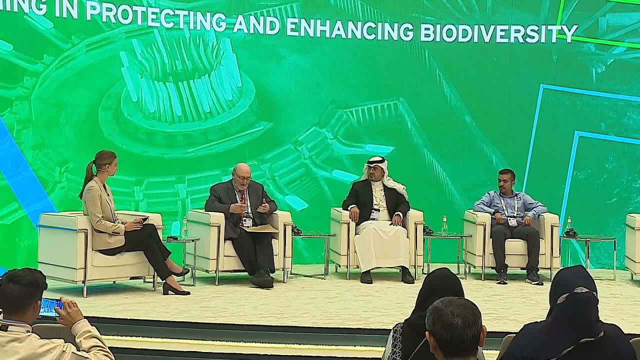 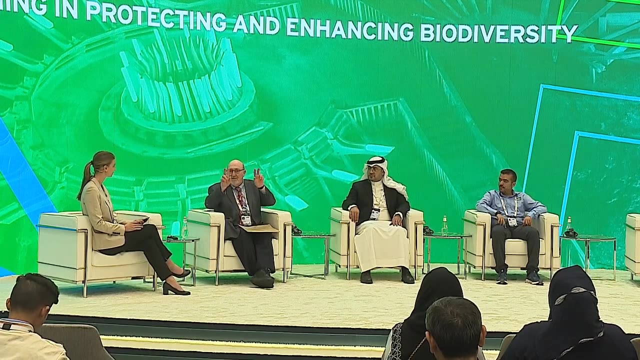 Considering the push to clean energy transition, how do you see the impact on communities and the environment evolving from future mining activities playing out on a global level? thank you, Catherine. the impact is going to be variable. so it's going to be variable both for communities and the environment depending on the mining project, but for the right mining projects. 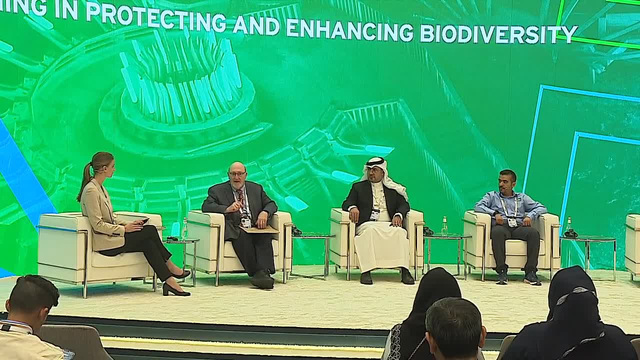 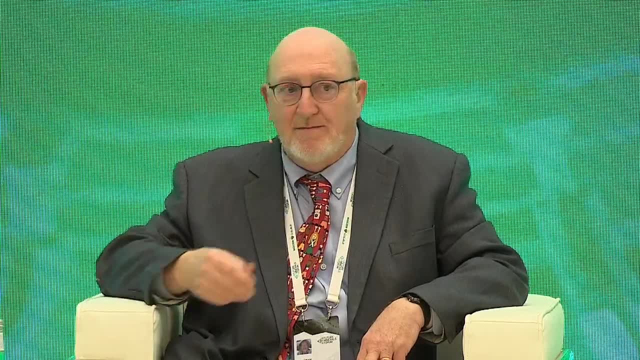 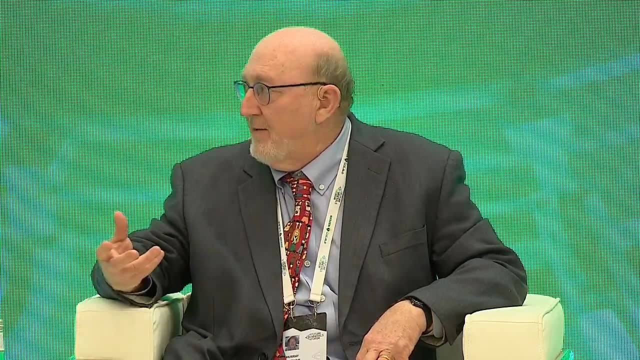 the ones we actually really want to go forward with. they need to have net very positive impacts in both those areas. so, in terms of communities- sort of impacts that people have talked about already today in multiple forums- increasing things like education, skills, economic opportunities- obviously- one that actually came up in an earlier panel today- 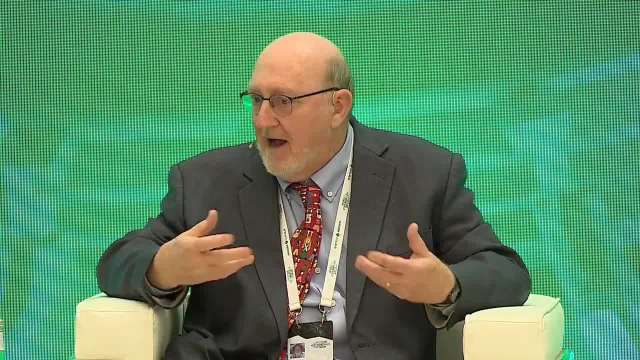 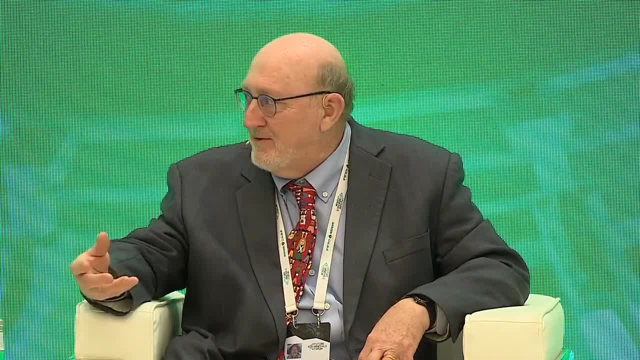 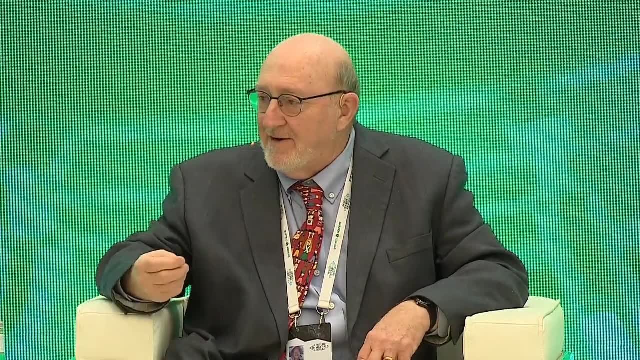 is leaving infrastructure behind after a mining project, for instance, now thinking about leaving renewable energy technology. so community has energy going forward that it didn't have before in terms of the environment again leaving to lead the environment a net positive, and that may be in ways like we're talking about in this panel. 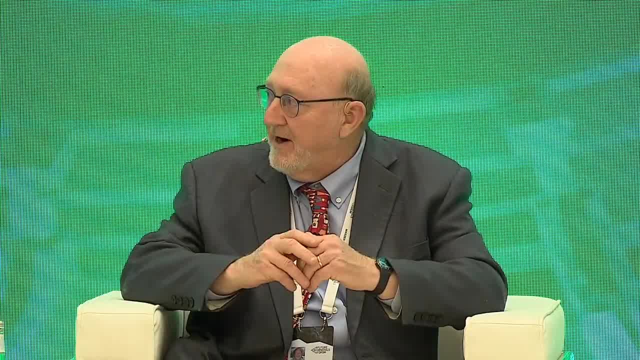 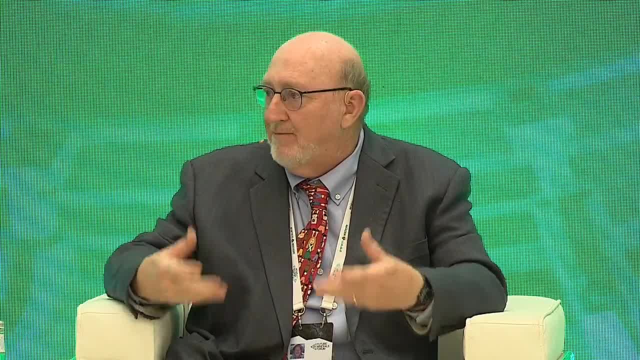 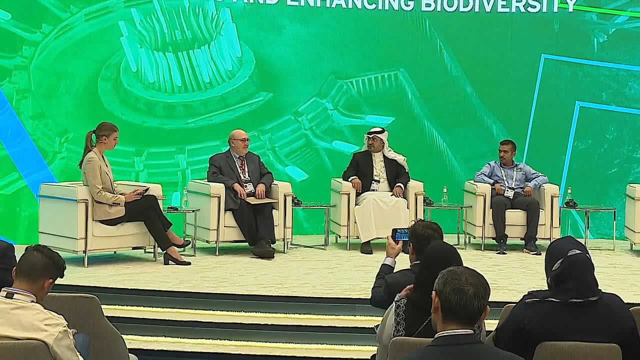 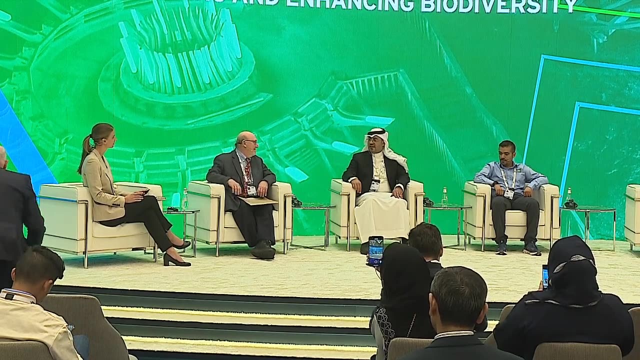 of increasing the biodiversity in a mining area or returning biodiversity that had been eradicated or impacted by previous populations being there before? thank you very much, Khalid. which commitments can a mining operator make to be seen as the welcome neighbors in the areas where you operate? thank you for a question. I would like to start really by the court, or quoting something from from. 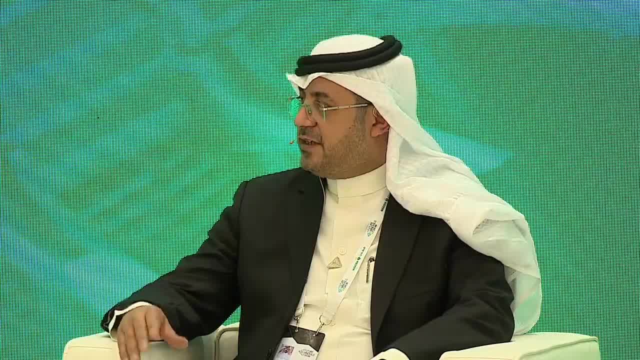 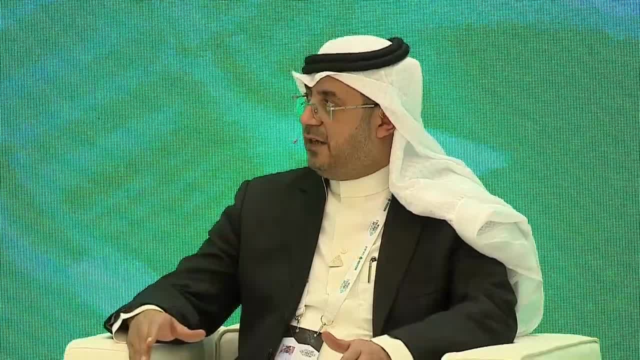 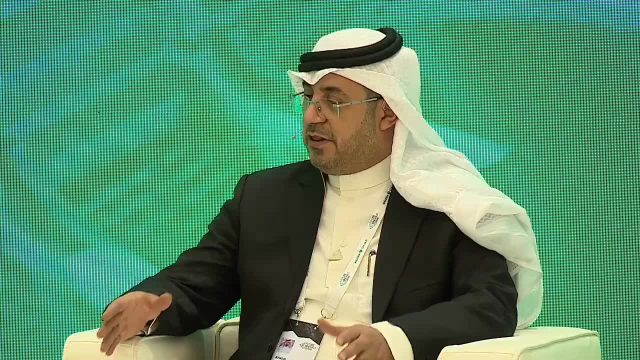 that opening session today. that's uh that uh, His Excellency the Prime Minister or the Minister Pender mentioned and highlights, uh yeah, money could be and somehow that's uh risking the environments and somehow, if it's not responsible, mining but on the other hand, mining is the solution really to save the environment. 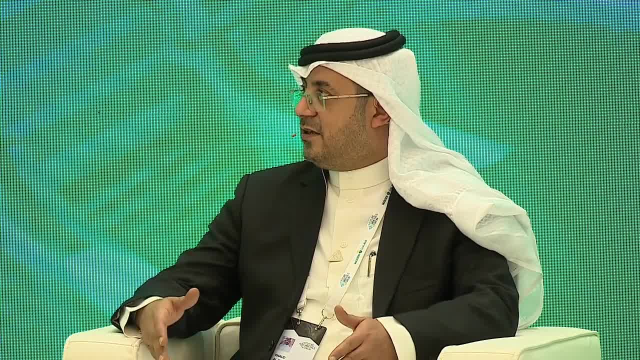 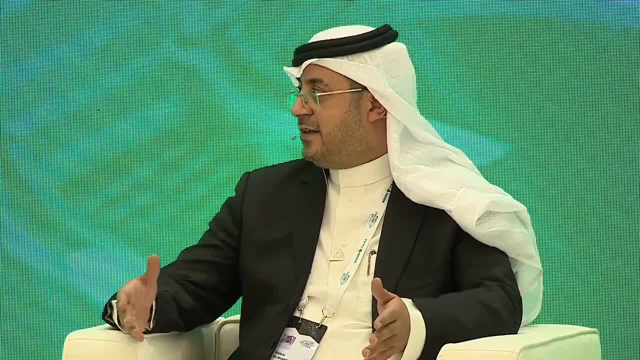 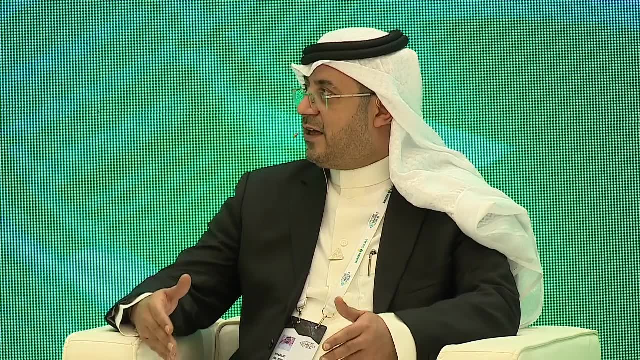 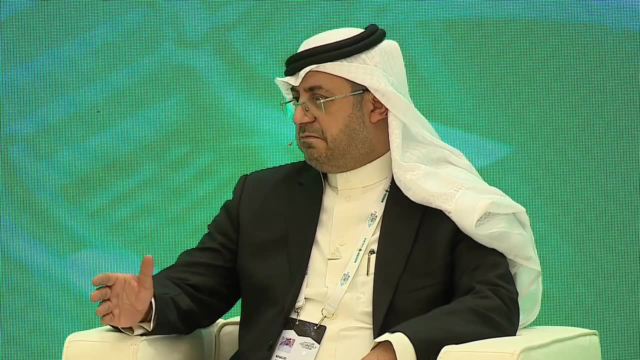 in terms of providing the right metals and minerals to, to, to build the, the decarbonization plant, uh solar panels and and and so mining, and somehow really is a right place to to, to, to, to, to utilize as a vehicle to build and maximize the environment in the coming Futures. uh, I think that, uh, going back to your 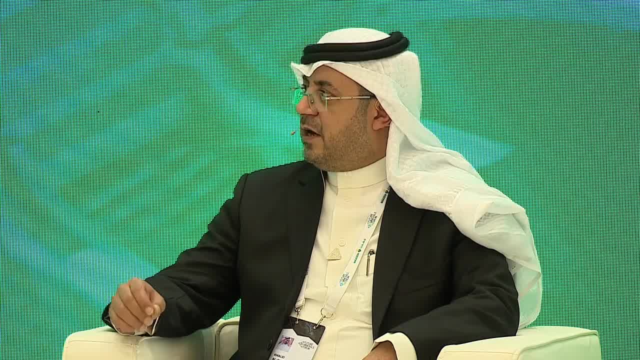 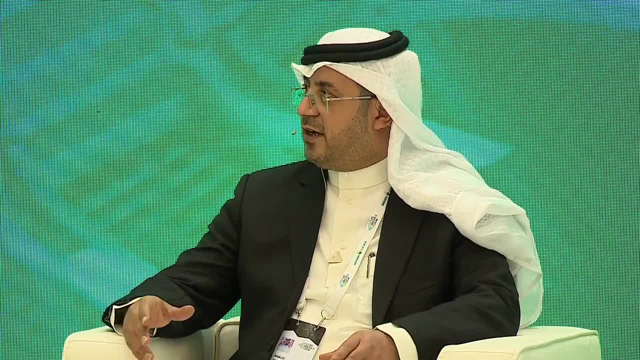 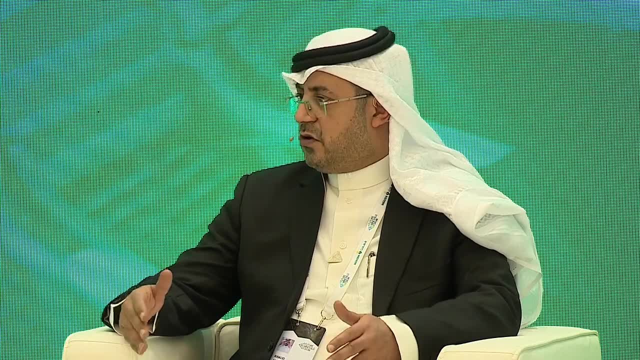 question. uh, I think the commitment that the mining need to do is is to make sure that they are not only a welcoming neighbor, they are engaging, really the neighbors, they are decision makers when it's come to to their place and, unusually, as you know, that mining usually are in a remote area. 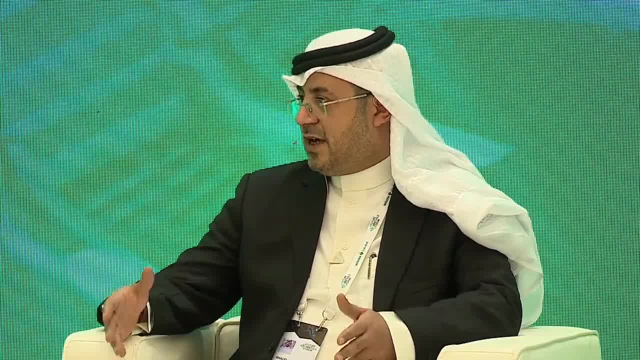 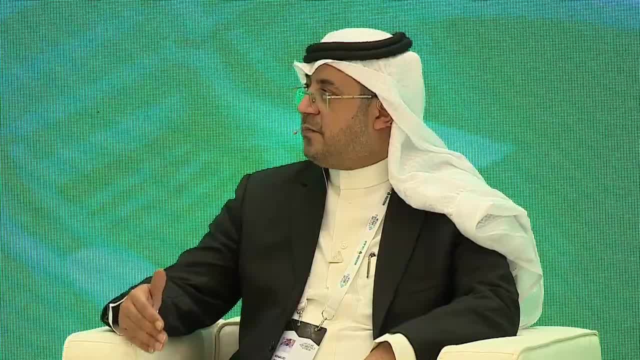 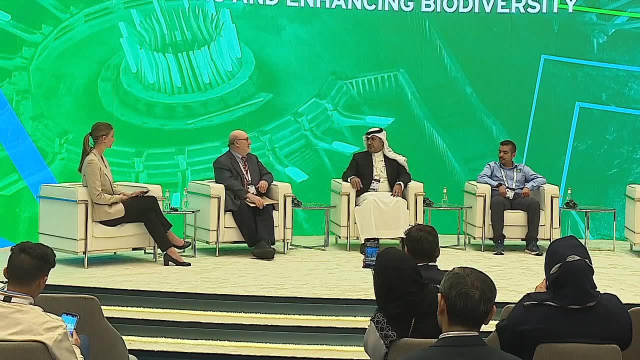 uh, disconnected area, less modernized area. so I think the commitment should be is engaging the commitment in their decision and providing the support whenever that is as possible. sure, maybe you can give us a bit of an example of what madden yeah, we have. we have been in in several places in 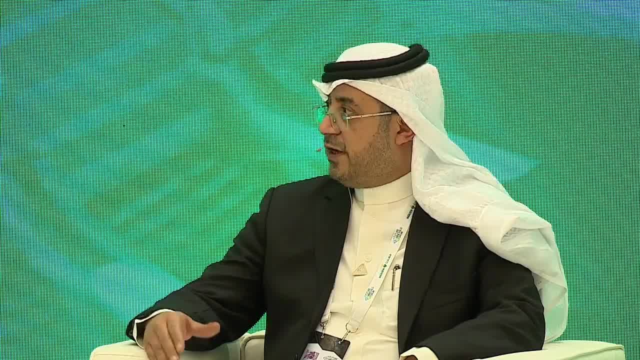 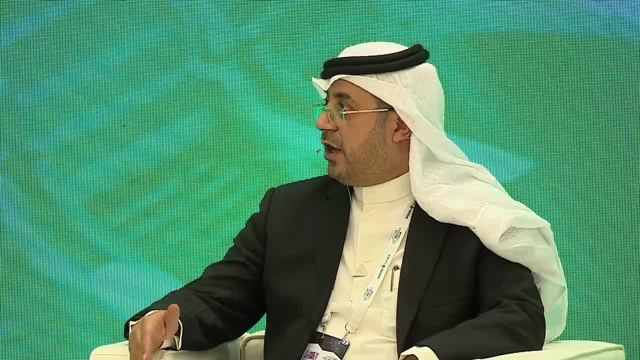 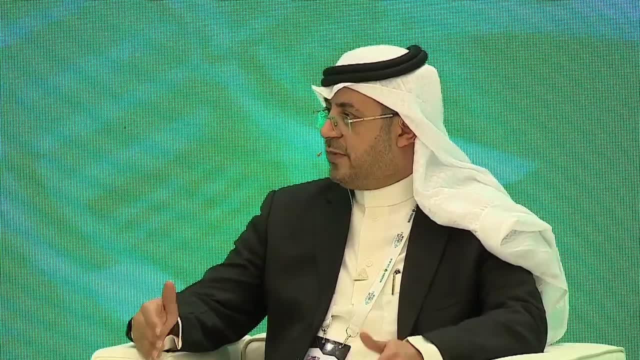 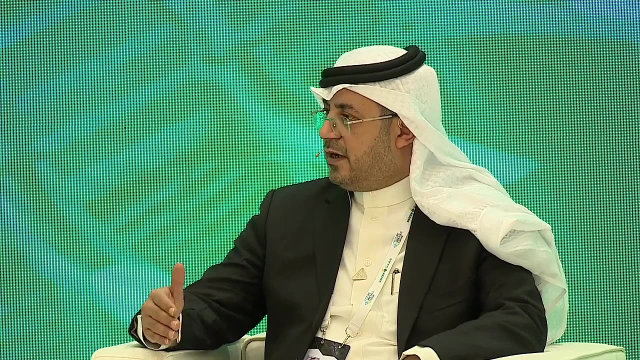 the region, for example, uh, the result of the engagement of the neighbor that resulted in building several schools, biotechnic College, where we are providing and preparing the future miners with, with the right responsibility, and then the one of our also operation that we provided so many, incentivized and and promote, even providing the the way that so 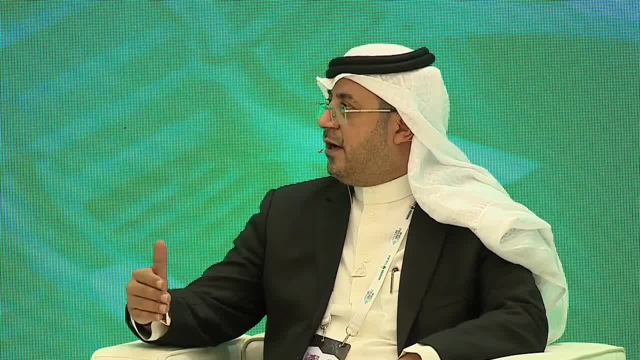 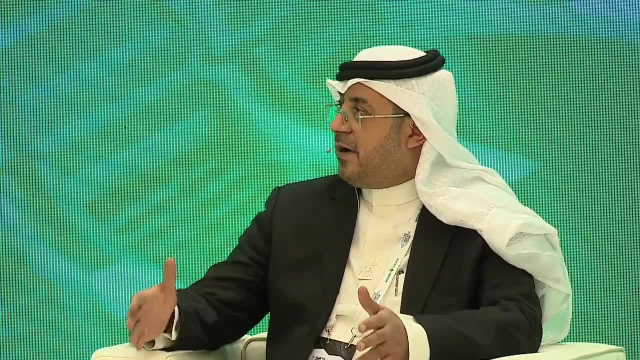 that the local, the females, that they can work in gold, and then so many others and make jewelries. So it's out of our operation exactly, but it's nearby and so many people that involved as an outcome of our operation Great. 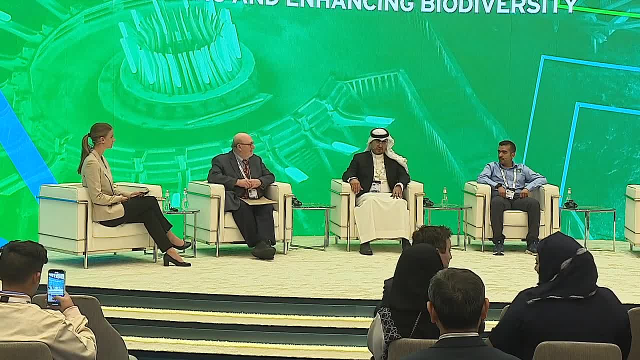 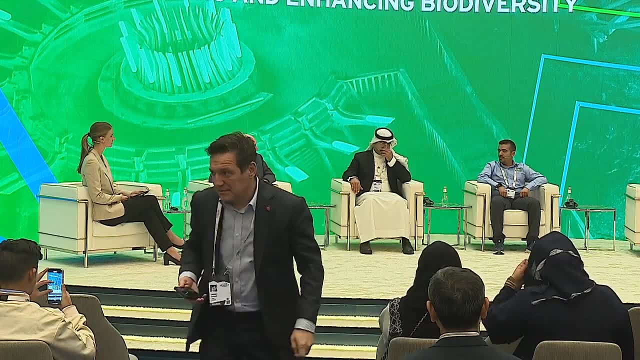 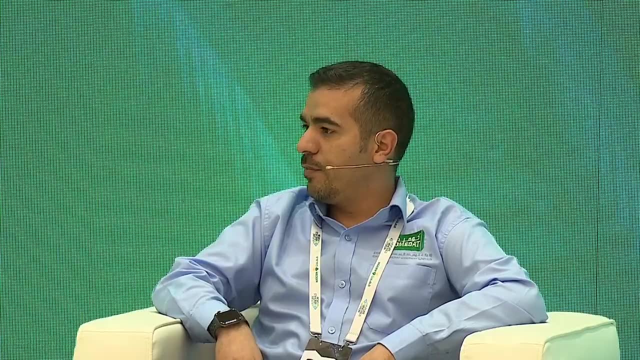 Hassan, how can mining benefit the local community where you operate, Actually in Saudi, the local community? for us it is one of the priority because we believe that for any mining succeed supposed to be supported by the local community And in our objective, 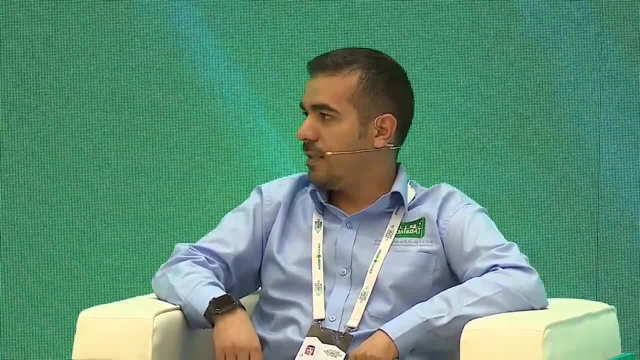 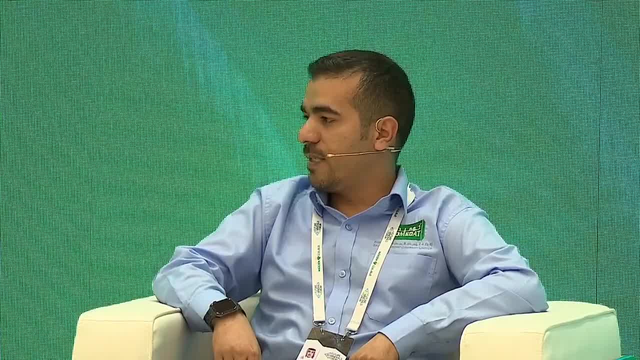 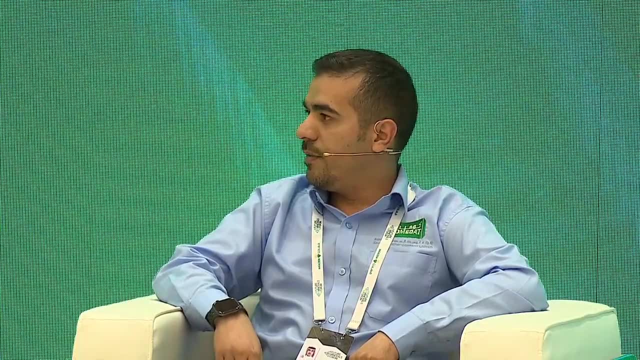 we have dealing with the local community as a partner to us and he's worked with us since we started. So because of that we are signing the contract with the Saudi Mining Polytechnic in the north region to train the people from the local community. 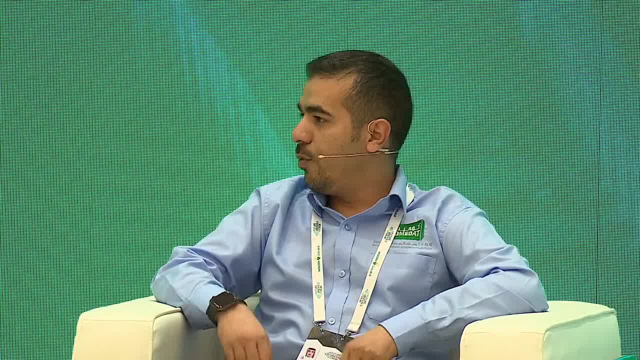 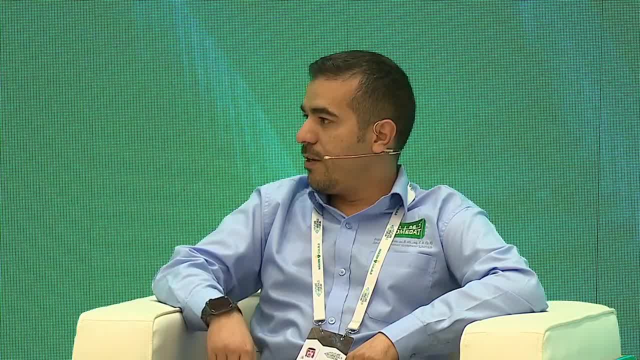 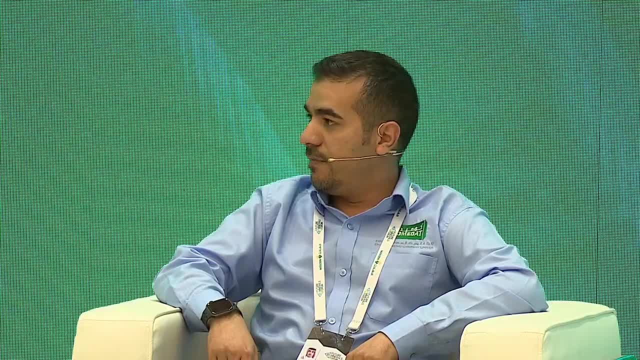 and this local community. at the end he will work with us in the mining. So, and recently we are- I am very proud about that one- We are the first mining company hiring the ladies and work in the mining field. So the local community, we believe it is. 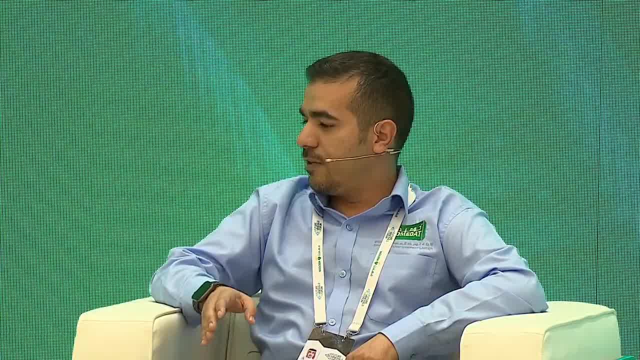 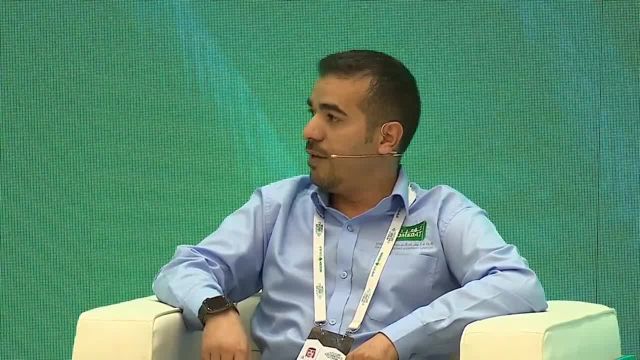 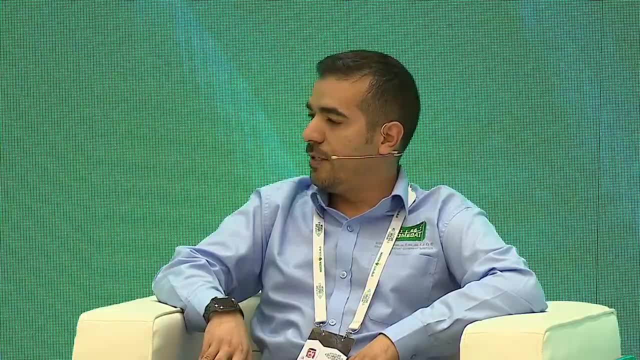 it is the main source for the human people in the mining, So this it will add value to us as well, Thank you. Thank you, As well as add value to the local people. This is from the human resource and the use of the local community. 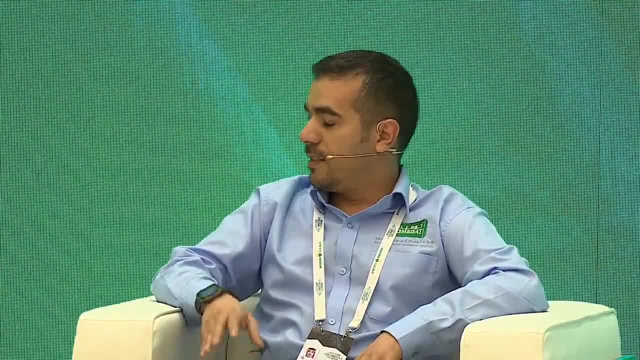 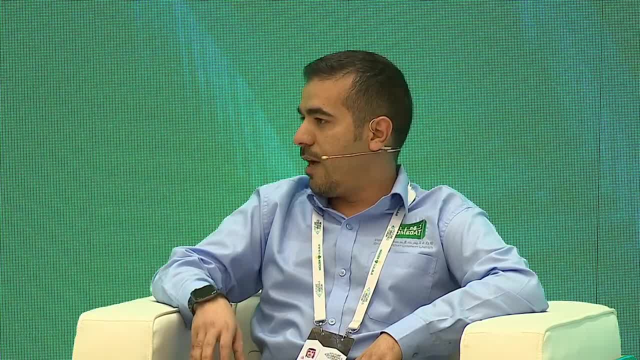 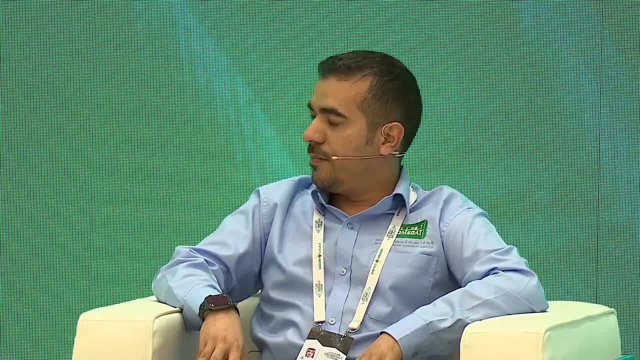 The other thing or other part. it is the supplier, The supplier of our spare part. normally in the mining, most of the supplier it is from outside. We import the spare part And last few years we replaced many of the spare part. 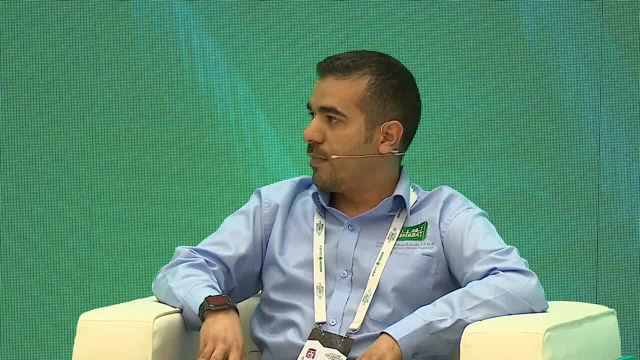 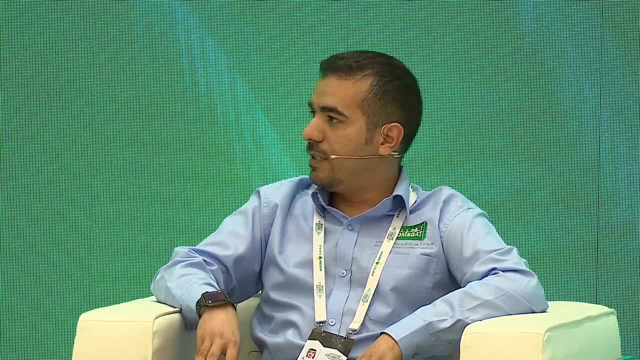 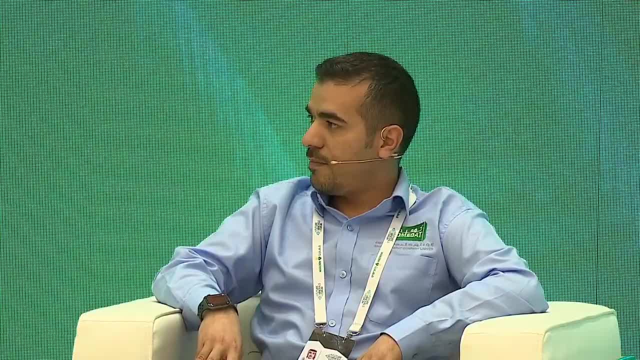 by the local supplier, which add value to him also and the income for the local supplier in Saudi. And this is it: help us to get our spare part early, as soon as we want that one Great. Maybe let's go back to you, Murray. 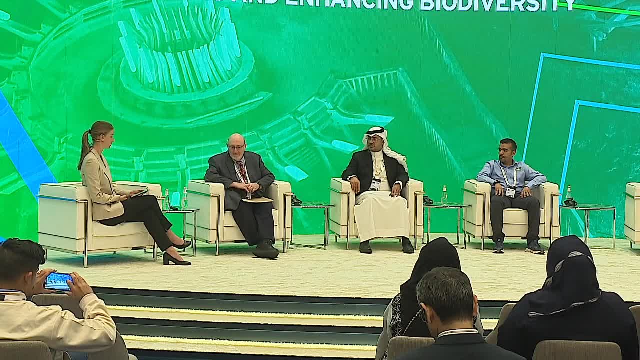 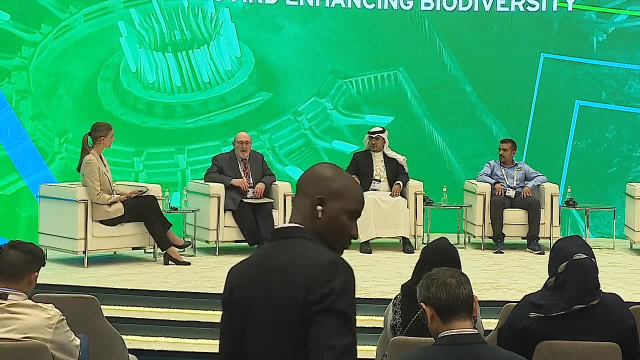 It has been said that geodiversity is required for biodiversity. Can you explain this concept a little bit, And why is it important for the mining sector? Sure I can. So it's a concept really from the ecologists And it makes sense. 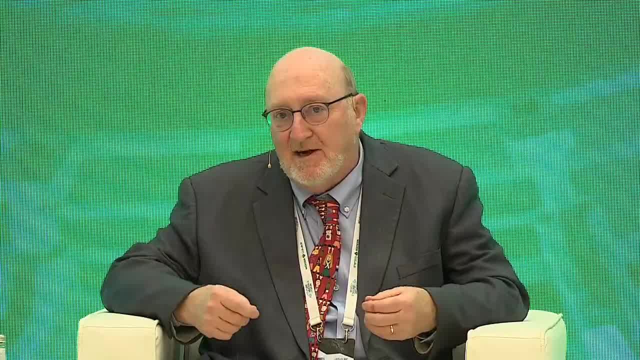 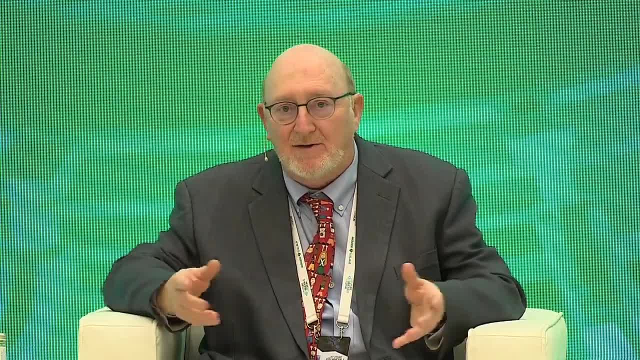 It's actually what we've been talking about at this conference: that our society, our civilization, depends on metals. That's what this whole conference is about. So if you think about any biological community, that's what we are right. They depend on what's coming from the earth. 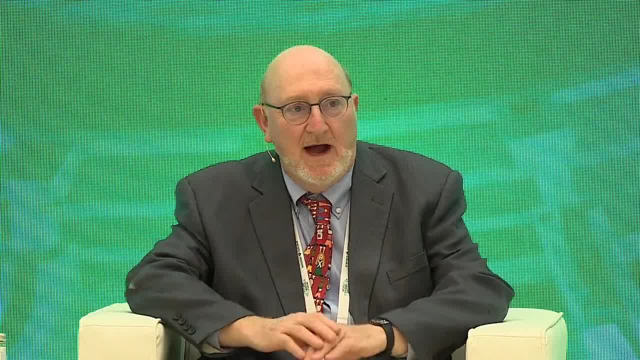 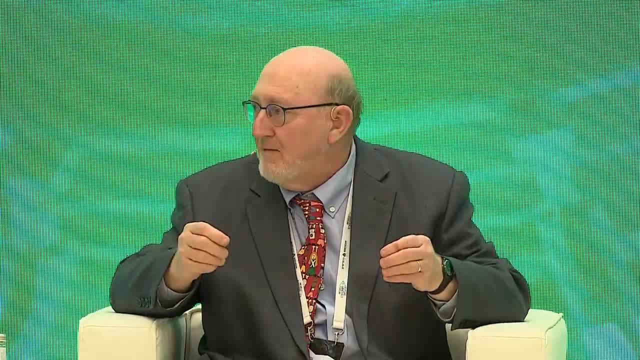 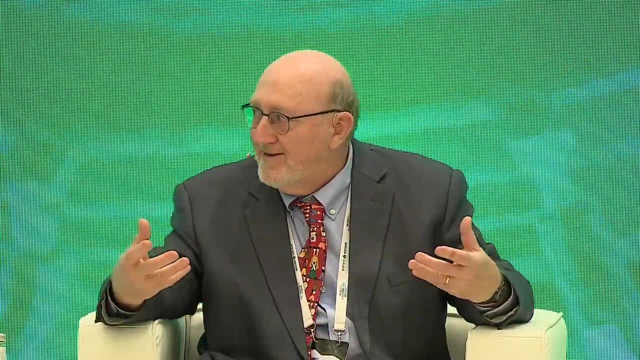 So geodiversity- what's in the earth actually determines what kind of biological activity can exist. This conference is just a sort of super example of that, But it's really important to get that across educationally to ourselves as an industry to understand why what we're doing. 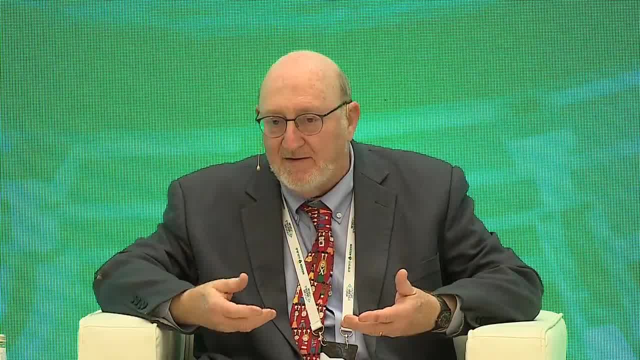 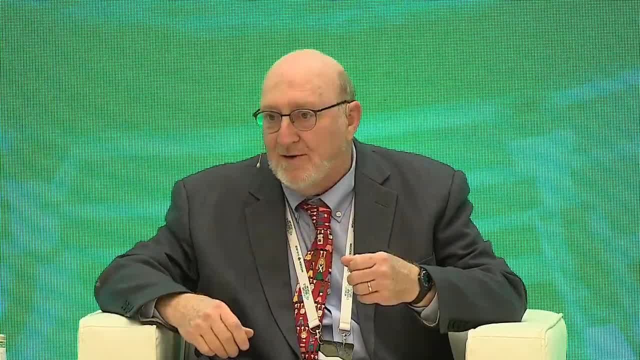 with the earth actually impacts all the biological activity and why we need to try and protect that, but also to society as a general, Because it again shows sort of the systems thinking we heard about from the panel before understanding how things are circular. 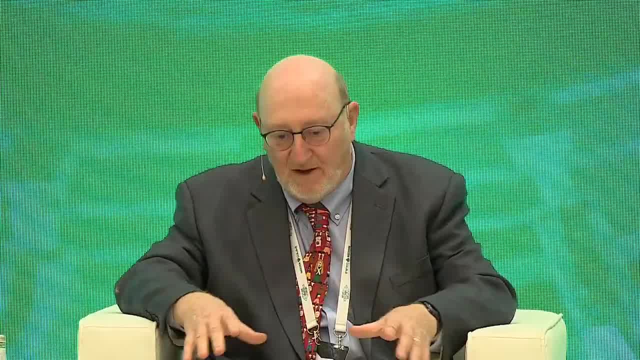 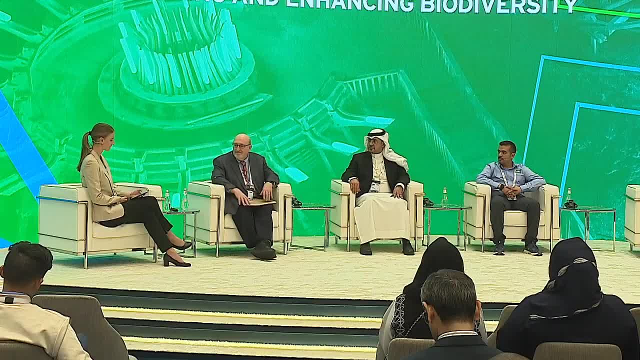 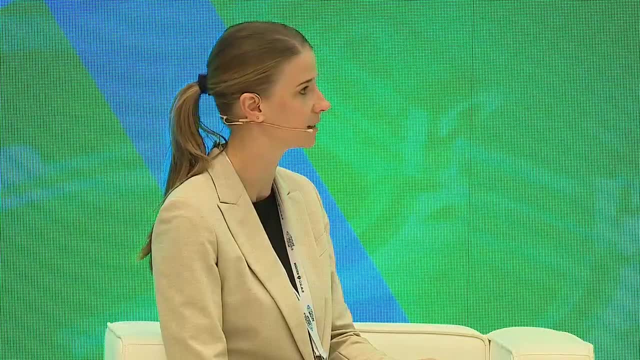 and how they're interconnected. So geodiversity, the earth- actually is the foundation of all the life on top of the earth. Khalid, what initiatives can mine operators take to protect the geodiversity, protect the environment, decarbonize operations? 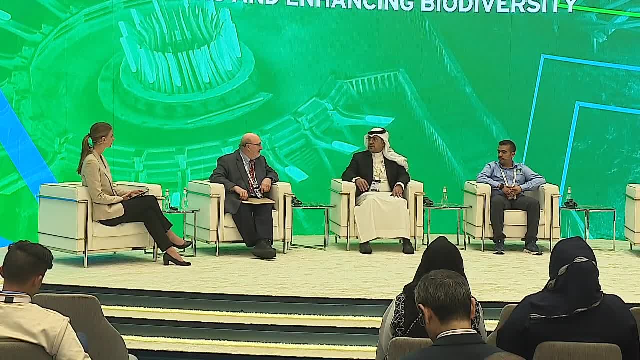 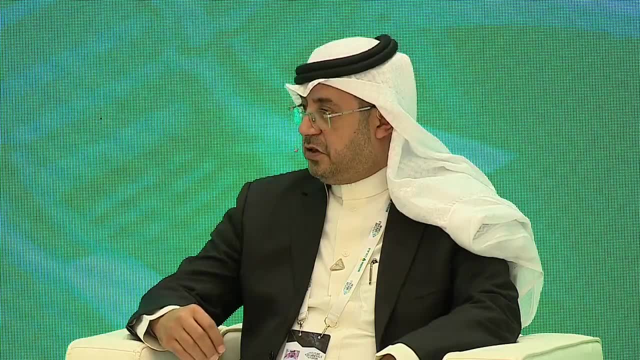 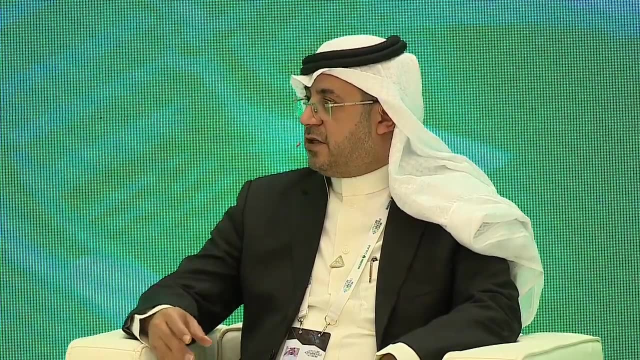 There are so many steps really to be taken, but I think one of the most important things is that efficient use of the energy and maximize the utilization of the renewable energy, renewable water that's for their purposes. These are the heart for any operation in the mine. 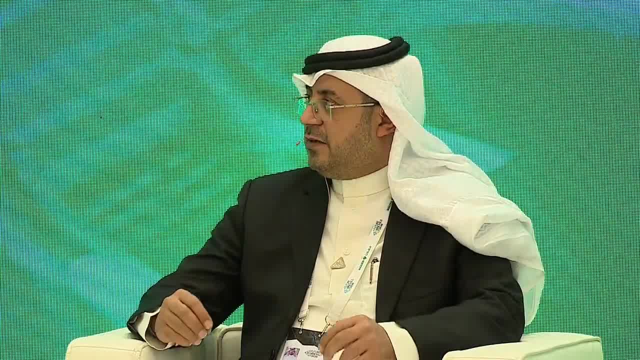 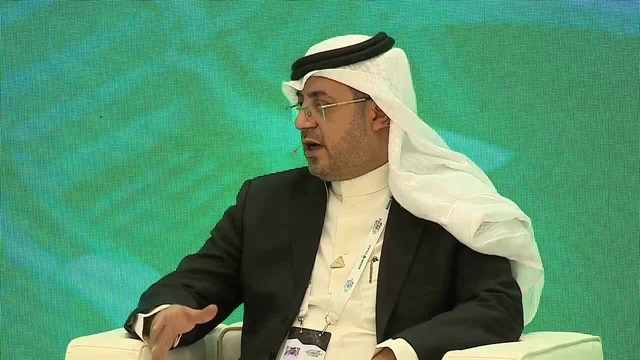 And then if we manage to utilize them in a more responsible way, that will help definitely Ma'aden, for example. we are now- we have just finished construction- one of the new operation and it's become one of the design criteria. 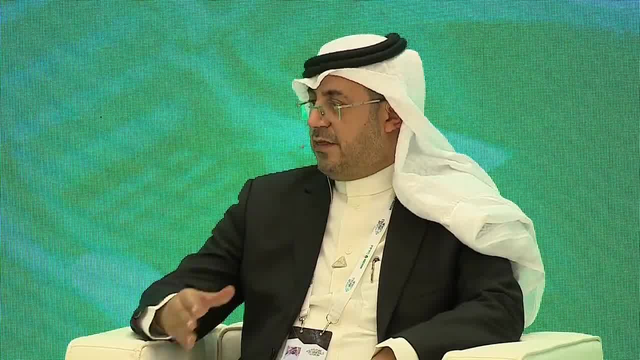 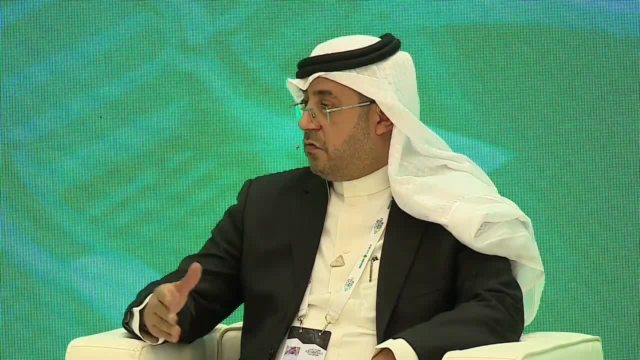 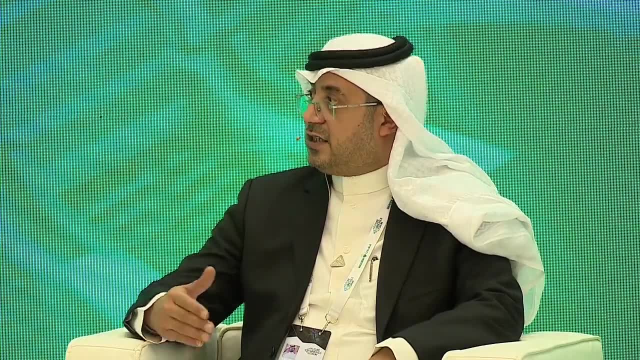 that to use the solar in our operation, And then that will be on as we build mines. we will, we will utilize the solar in our operation Water. we have, I think, built so many examples in utilizing the recycled water in our operation. 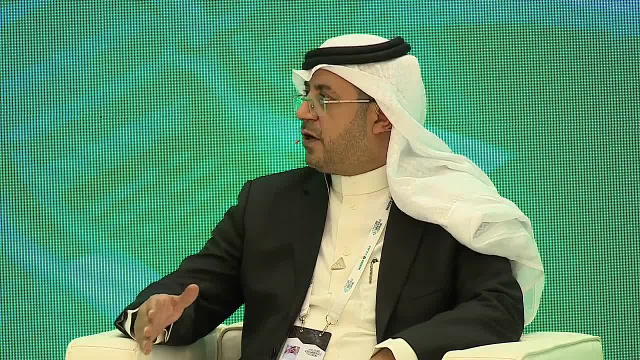 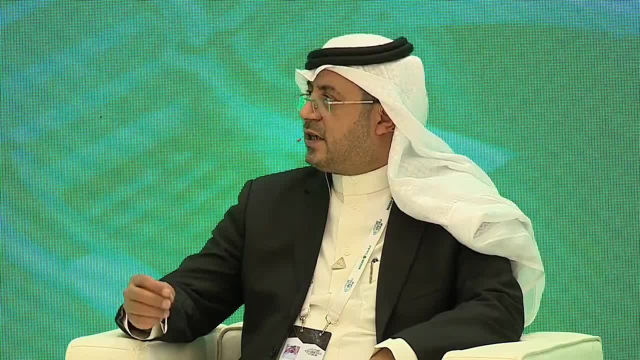 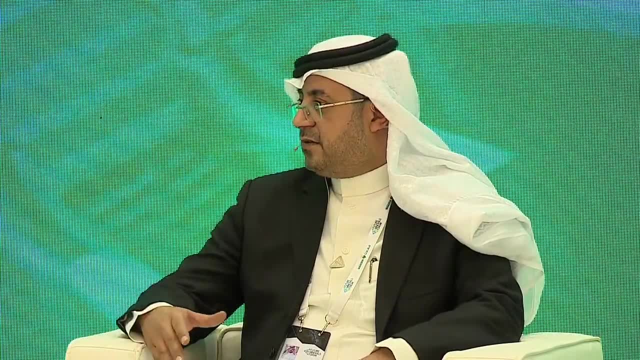 So, for example, in the past three years the average almost of our utilized water or used water in our operation and in the gold, for example, we have exceeded 65% of our gold produced. that's coming from utilized water. We have built more than 1,000 kilometer of pipes. 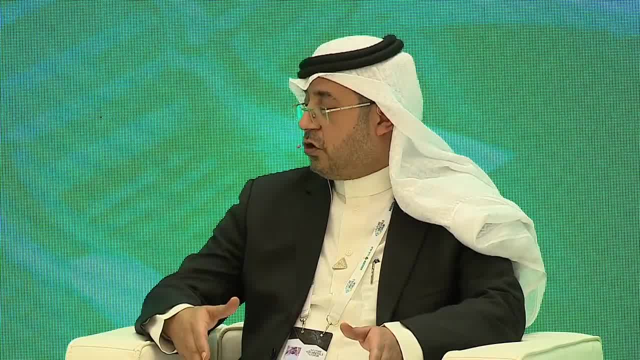 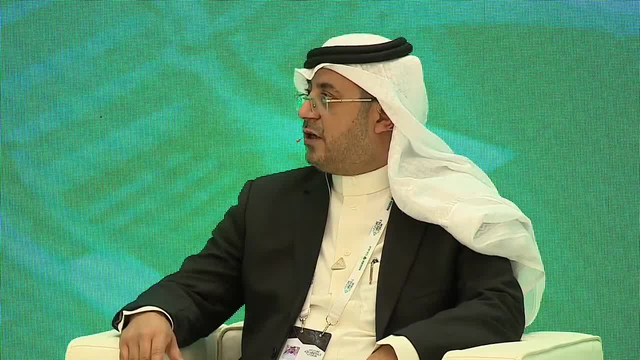 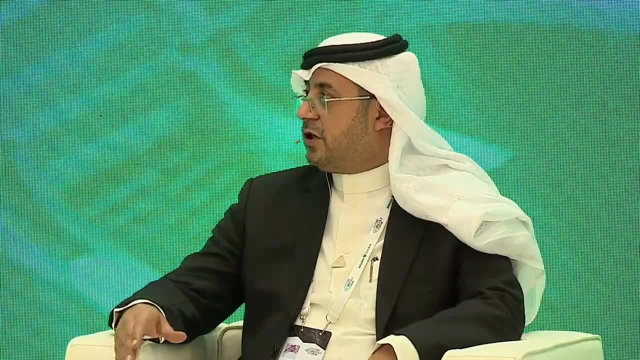 to provide our operation neither to the gold operation or to the north operation in the phosphate company with the recycled water, And we are aiming, in the phosphate, to jump from 50% of depending on water or groundwater to 100% of utilized used water or recycled water. 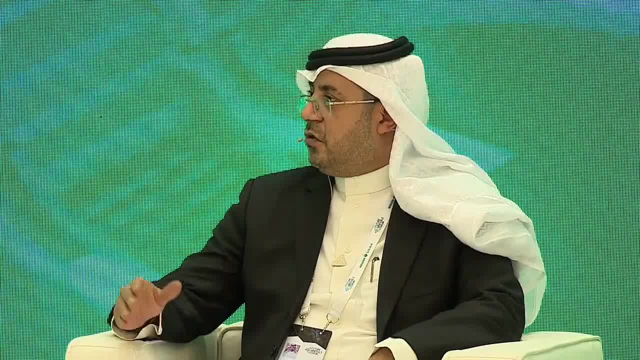 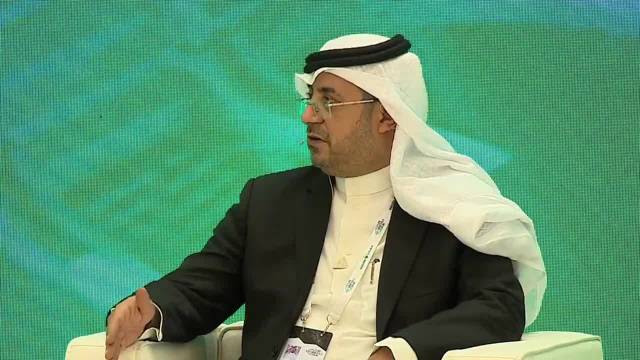 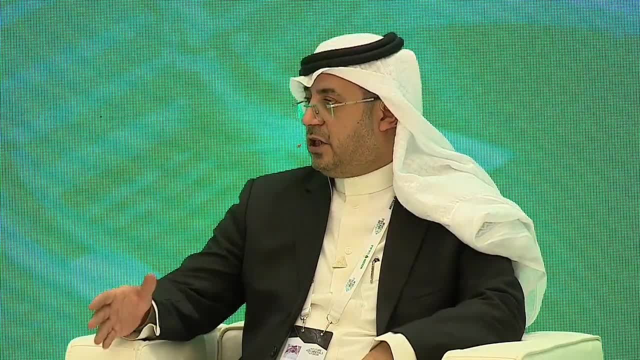 Similarly in the used water. We are working with so many government authorities to maximise really the use of the treated water in our operation, which is, I think, these are the two main really parts. In addition to this, of course, mine always knows as a waste and there is a waste material. 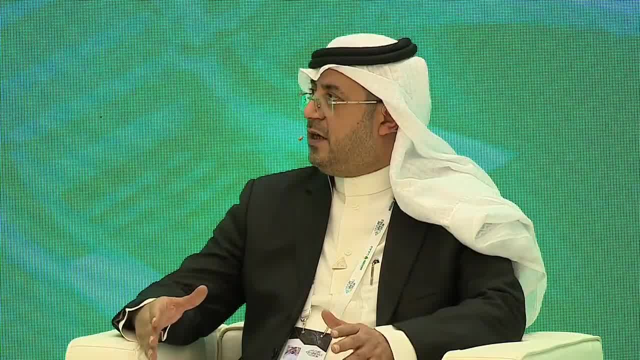 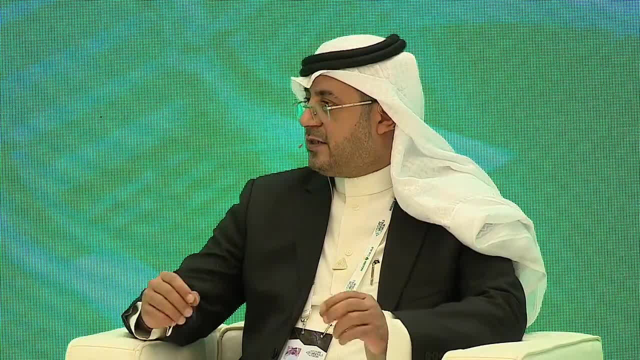 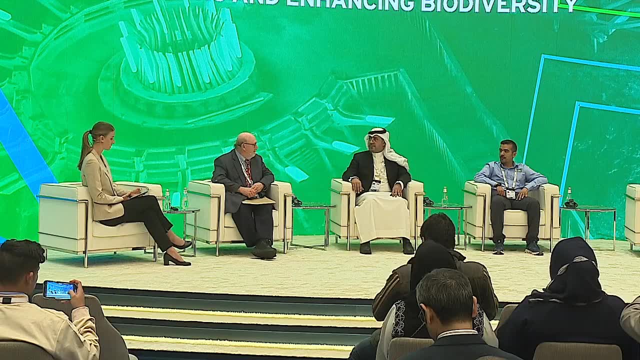 I think the main point here is to design this waste material in the proper way, in the right way, as per the best regularity or best, let's say, policies to keep this waste safe and protected throughout the time. Sometimes it's not possible to make everything as perfect, as Marden is doing that and conflict. 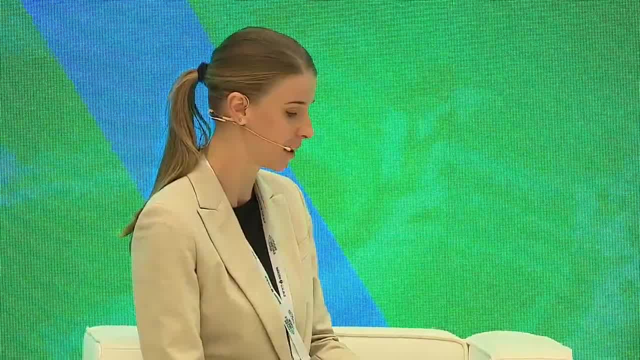 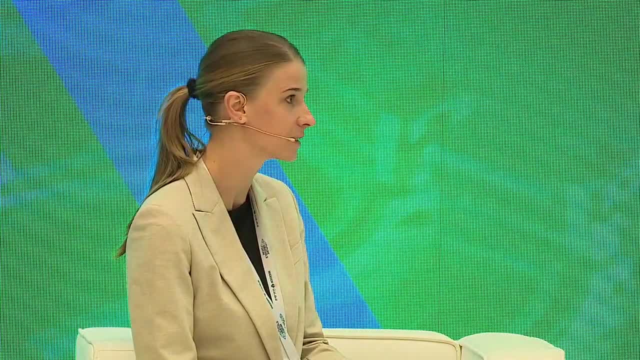 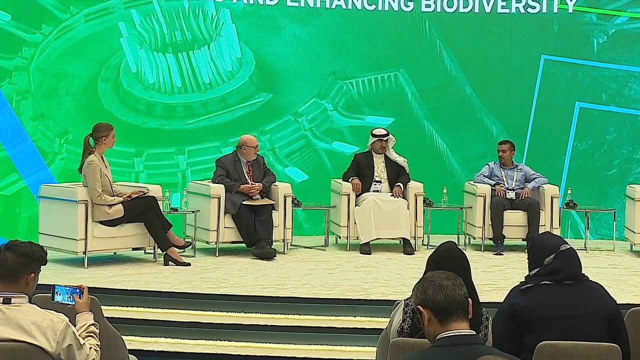 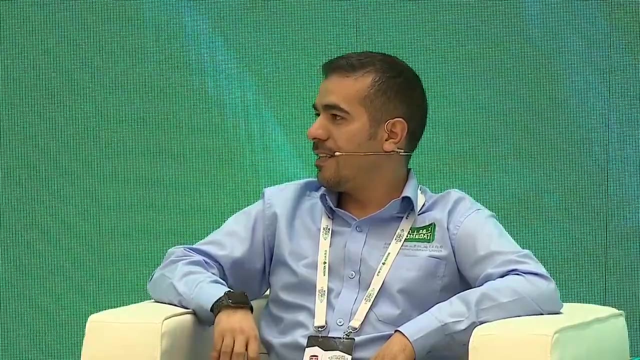 might also arise. Hassan, maybe you could say how mining operators can deal with social and environmental conflict, how they can deal with it. Actually, when we mention environmental or the mining, when we mention to anyone, the first thing he will thought or he will think it is the mining, it is disturbing, the environmental. 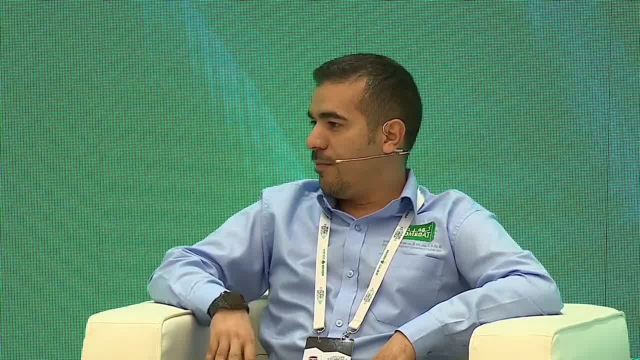 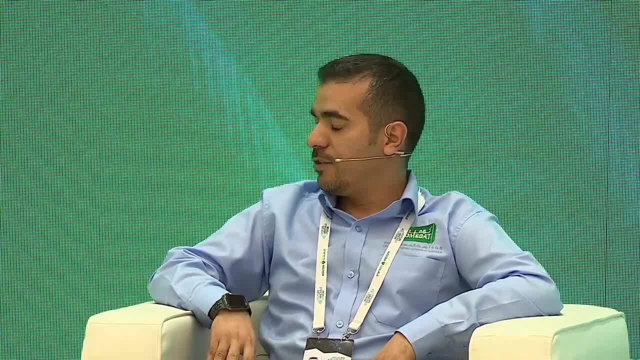 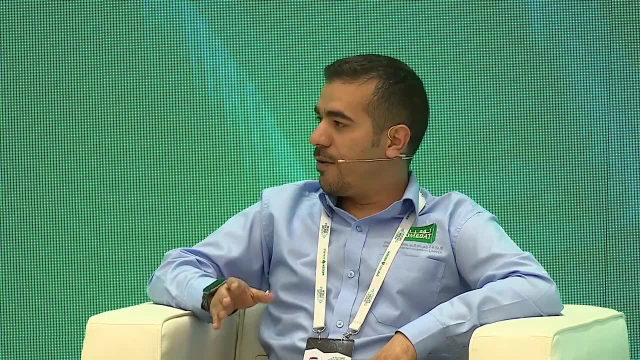 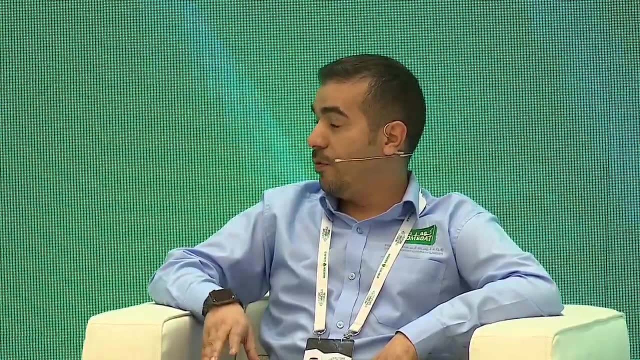 and the area. But where I am working the phosphate mining, we put the environmental thing. it is priority for us. So this is why we are dealing with the environmental very carefully, Very carefully in that area. We have our own weather station which can read daily and hourly the reading of the pollution. 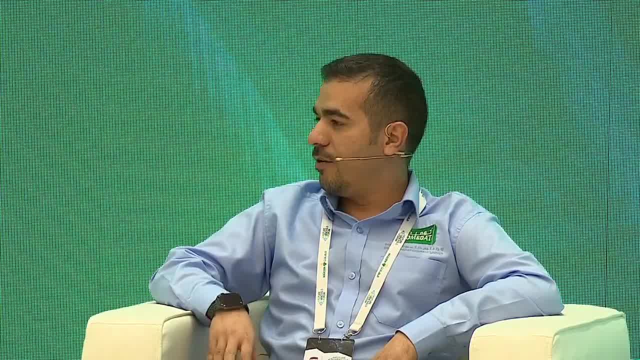 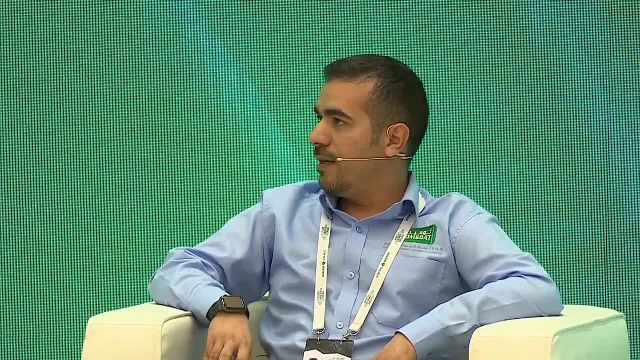 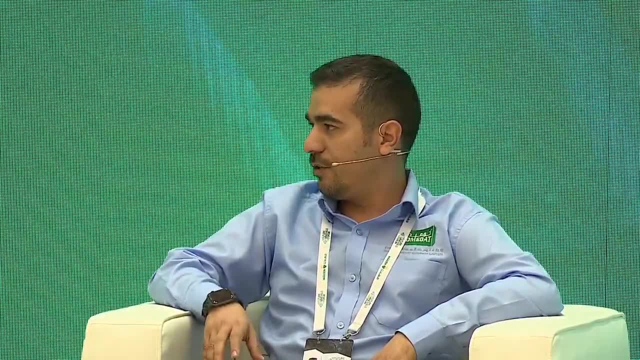 in the weather. Other thing: the recycling or disposal of the used tire, because we know there are many things came out from the mining: The oil usage, it is a lot, It is a huge number, And the tire also same thing. 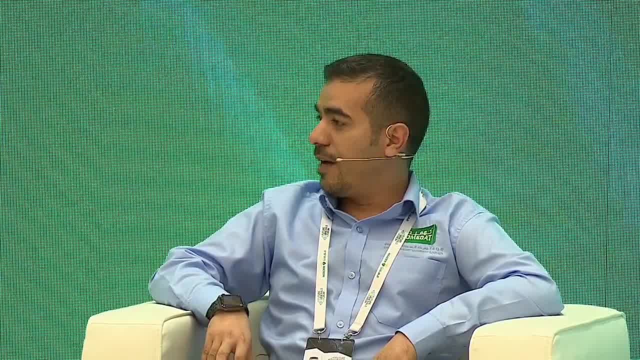 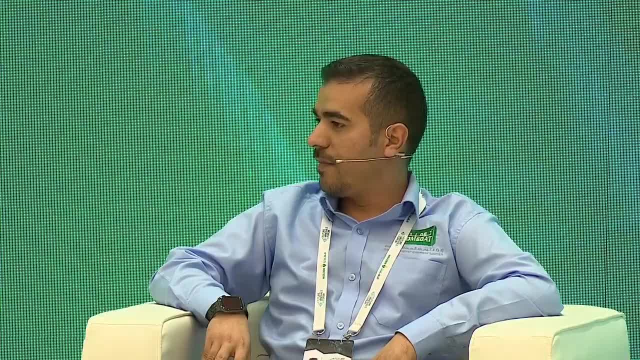 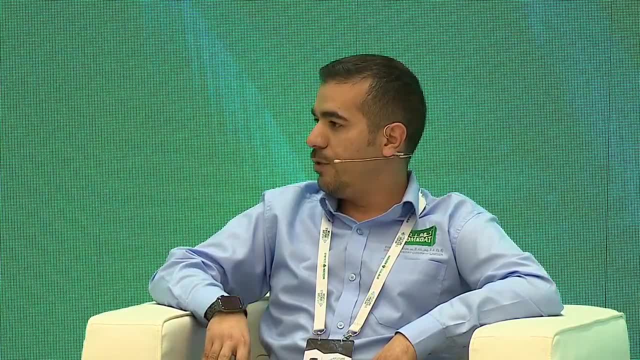 So in this thing we are dealing with authorized contract to disposal the tire and recycle also the used oil in the mining. Addition to that one, we are using the water treatment to recycle the water- what we use, and we have plan also to build our own sewage water recycling. 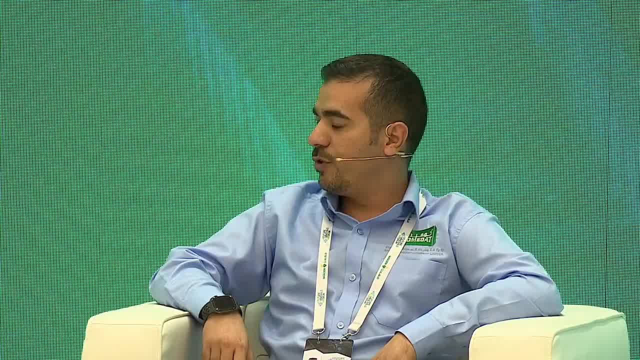 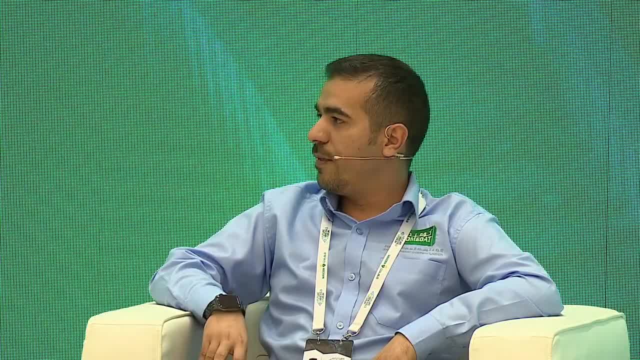 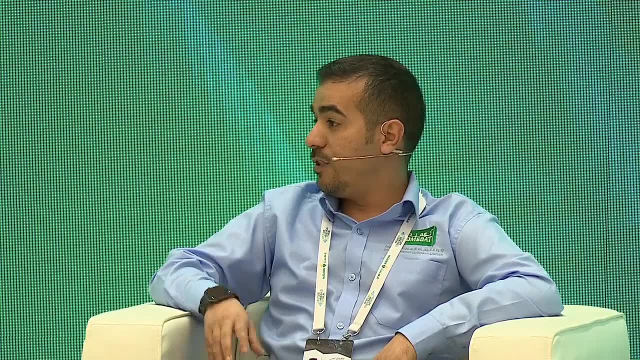 To reuse the water, To recycle the water. So we use the sewage water for spraying the water in the mine. We use also the water which came out from the process plant in Maadin to use it as suppression system inside of the mine, which will lead and it will help us to have control of the 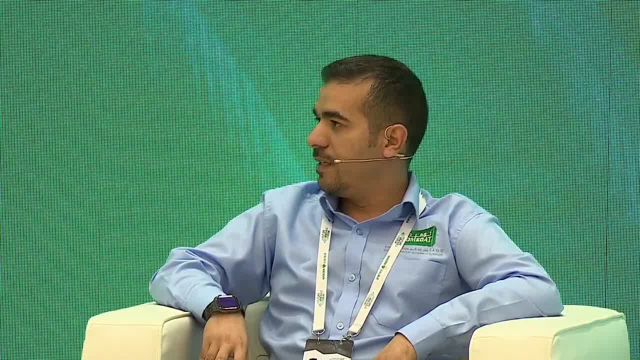 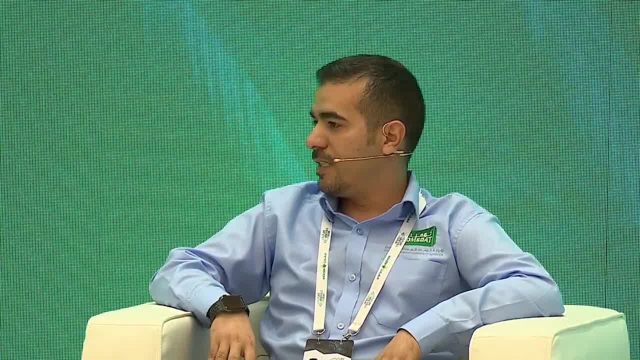 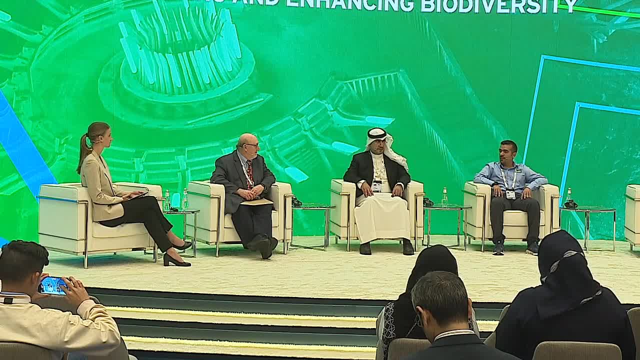 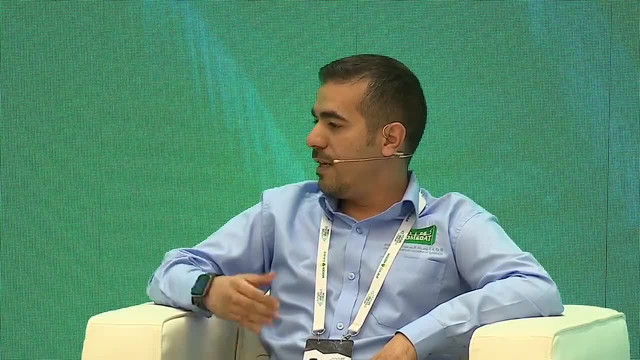 And if we want to link to the first question to make, and he don't have that threat about the mining, it will effect his health or it will affect the environment. Also, in the open bit we use the in-bit dumping, which means that same material, what we are. 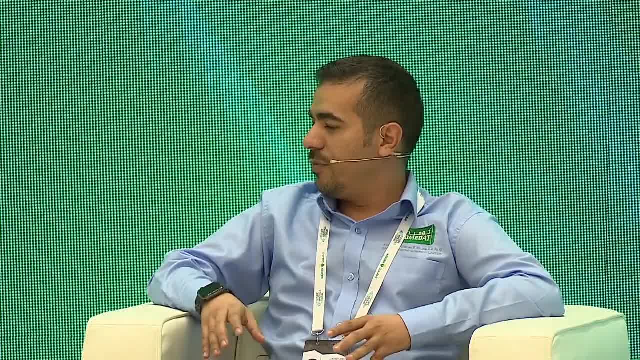 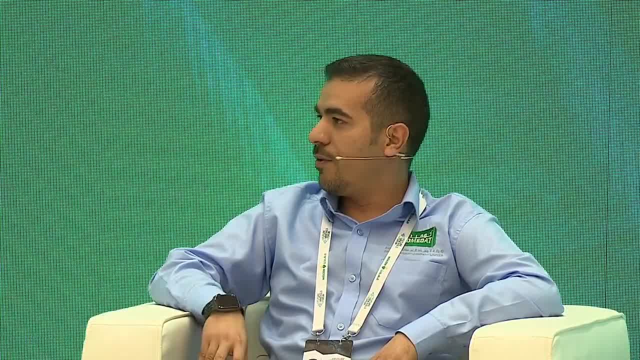 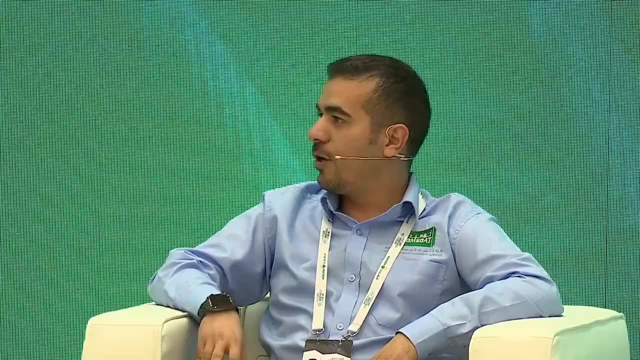 extracting, we dump it inside of the bit, which will make more control and the dust can be treated there. Grand, sad to you, justач dust in the local area or in the town around the mining, and this is it. help him and also it help us to make the local community and the people around happy from the mining. 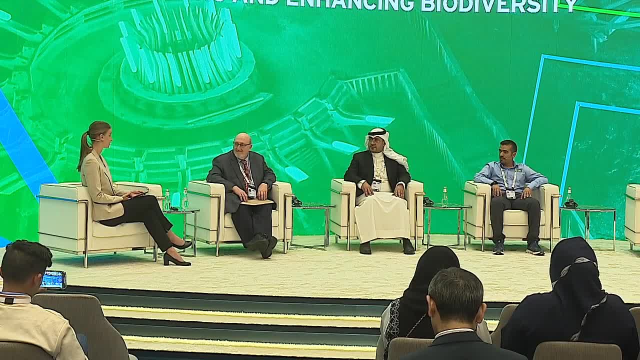 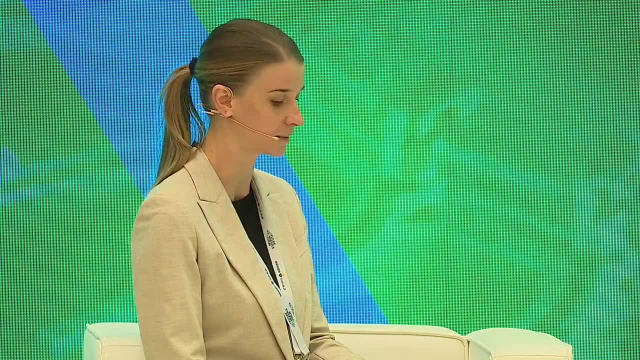 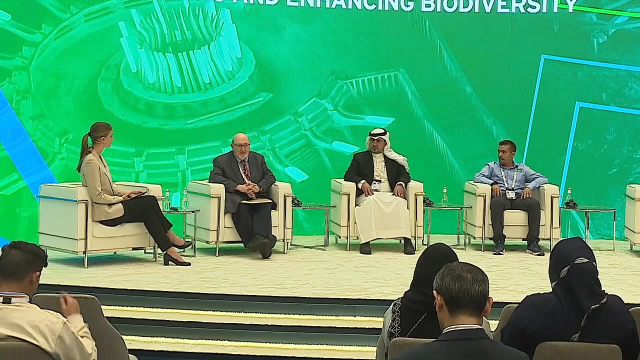 That's great hearing so many great examples from the Kingdom of Saudi Arabia, but, Murray, maybe you can also tell us a bit more about some examples of mining projects where biodiversity has explicitly been addressed and successful on a global level. There's actually a number, and I'll just mention three fairly briefly: one from Ireland where 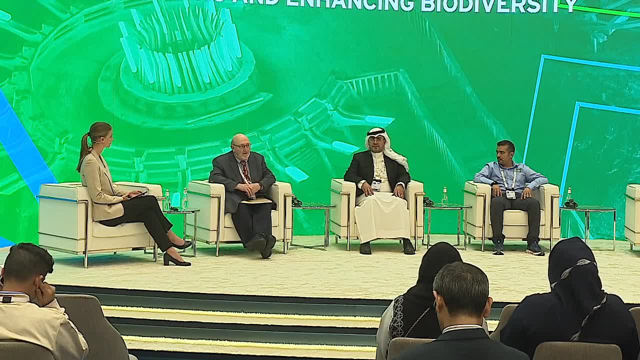 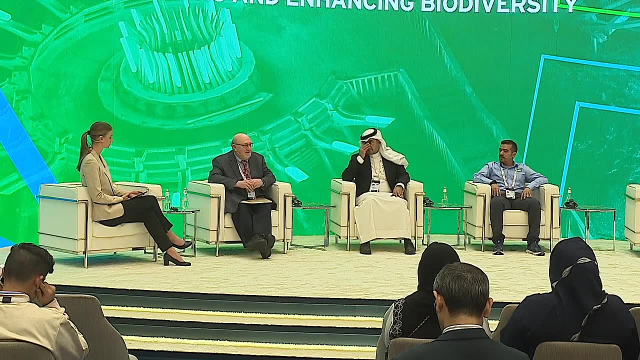 I'm from and mine there, Galmoy, which closed several years ago. actually, its tailings facility was engineered to be a wetlands, which has now been demonstrated by a number of nature groups in the country to actually have some of the greatest biodiversity in Ireland. so 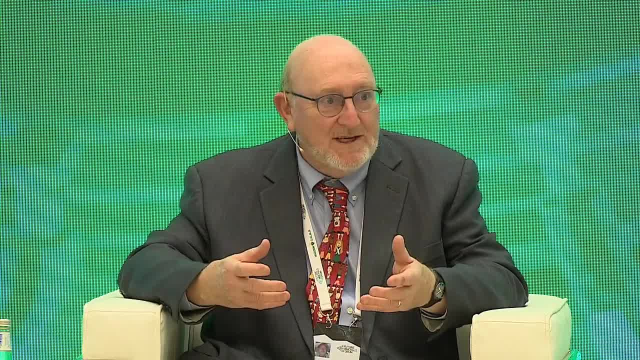 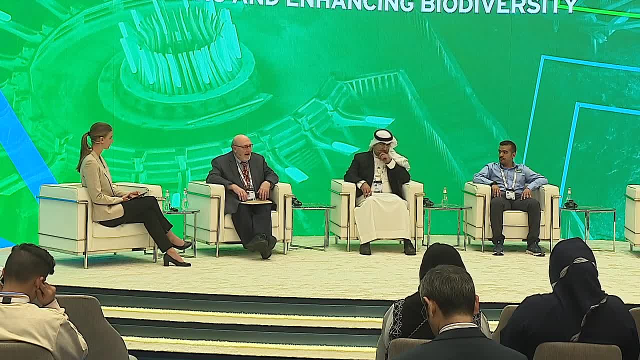 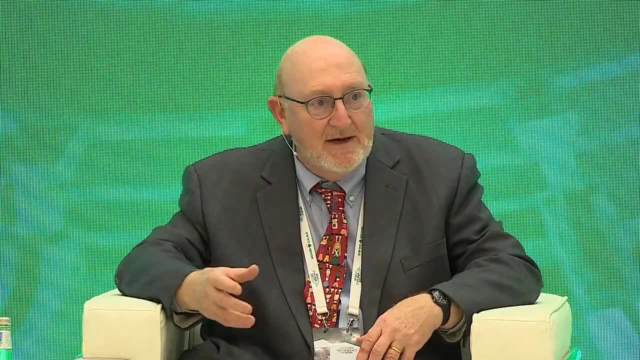 pretty amazing to take a manufactured- Yeah, What was a tailings facility and make it a center of biodiversity. I also do a lot of work in southern Africa, and there I'd just like to call out one company in particular. first, quantum. they actually take their mining sites in both Zambia and previously in DRC, and 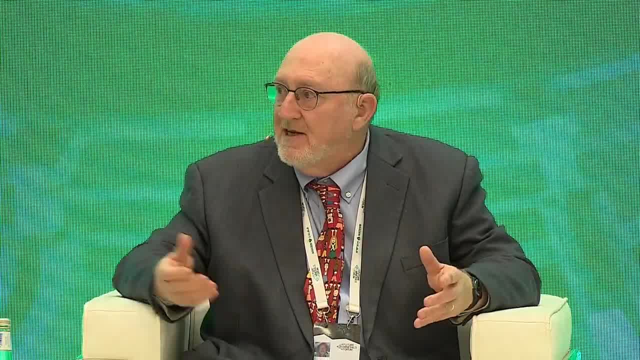 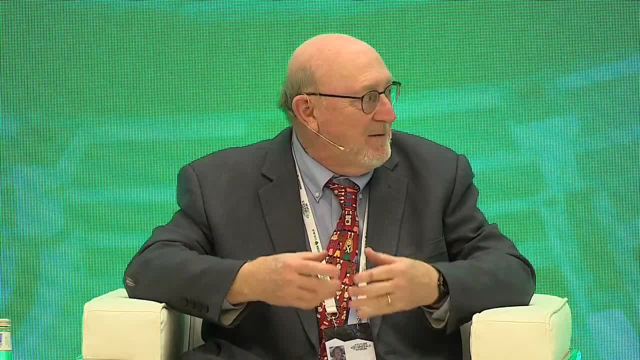 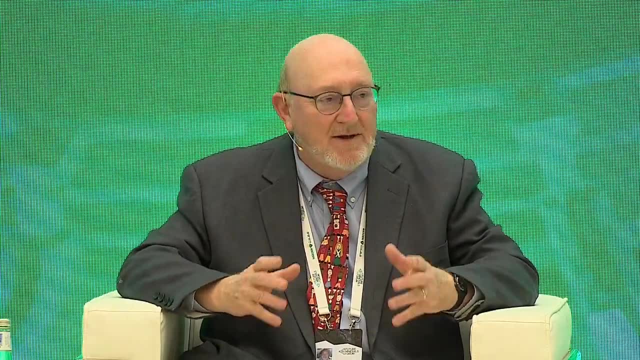 they've actually turned them into biodiversity oasis. they have reintroduced animals that were completely hunted out before, and so now the animals are back on the mine site and it looks like the way we all think Africa should look. The final one is probably the biggest, and that's the cars us mining district in Brazil. 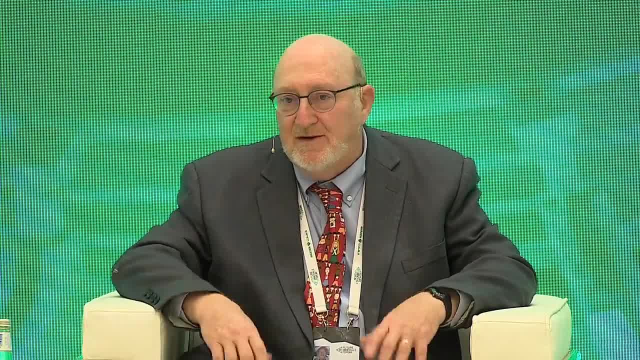 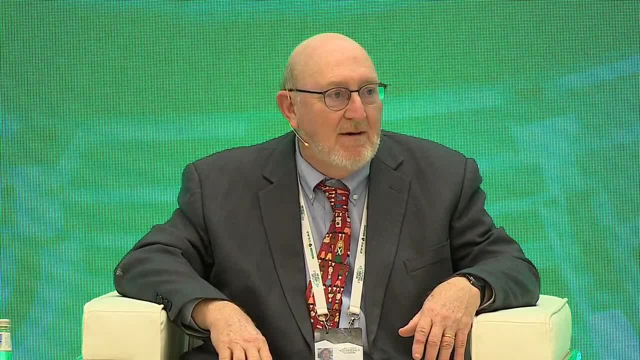 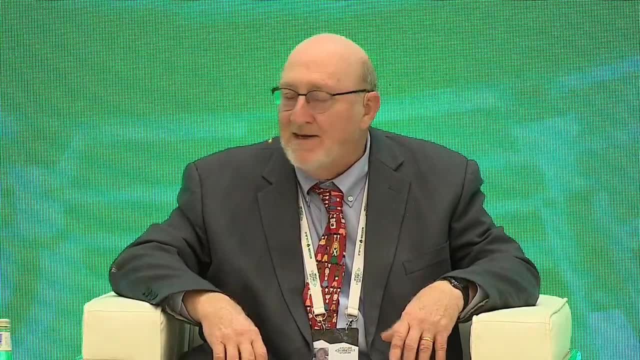 If you go to Google and go to eastern Brazil, most of it you can see there's no, there's no forest left, but there's a big square and that big, huge square, which is several hundred kilometers, is actually the cars us mining reserve which the government put in place back when it was all forest. 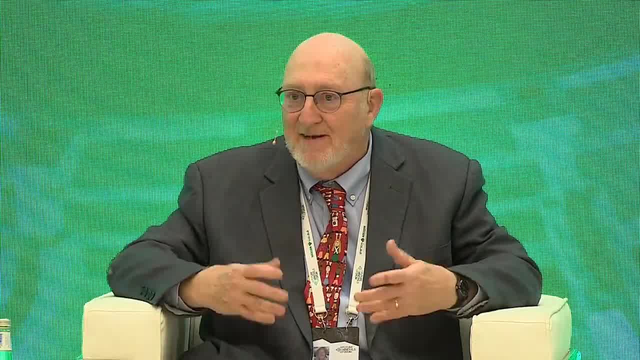 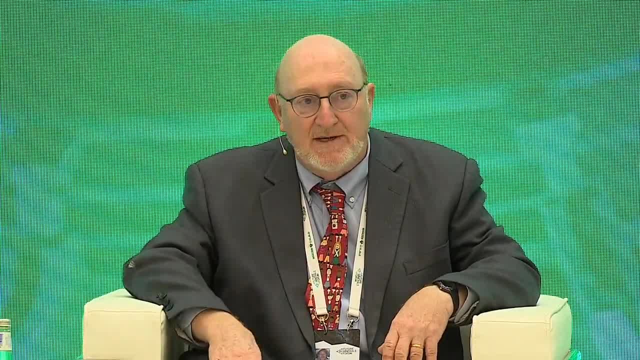 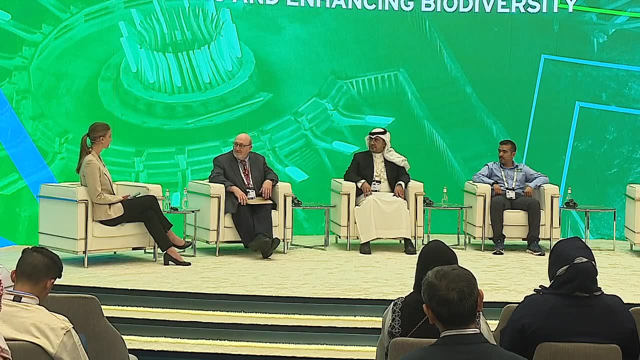 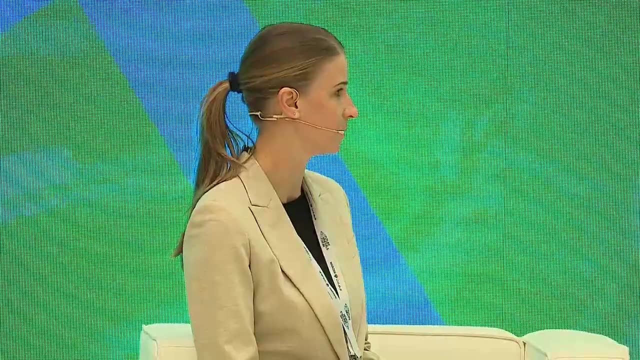 It's now the only part of the Brazilian Amazon that still is forested in that part of Brazil, so they have definitely preserved an incredibly important piece of biodiversity and the environment. That's great. Maybe more some some more examples of what modern is doing, not just to minimize the impact, but also to really encourage ESG principles. 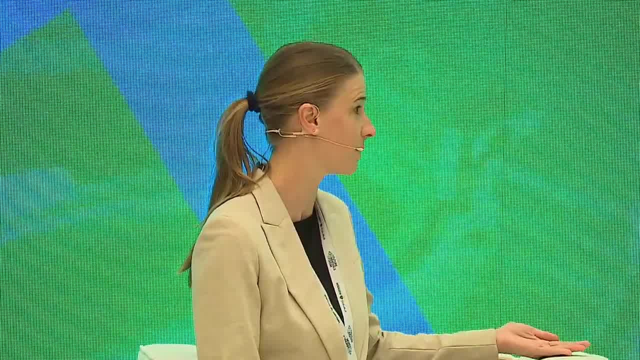 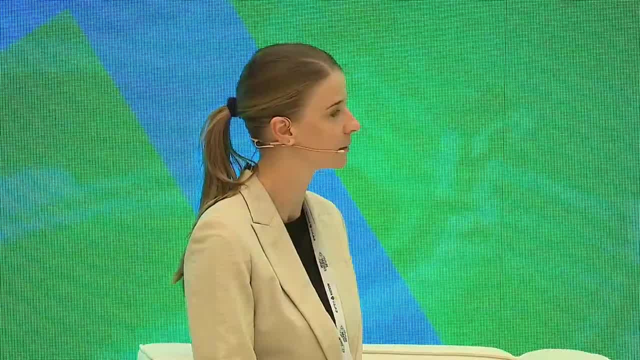 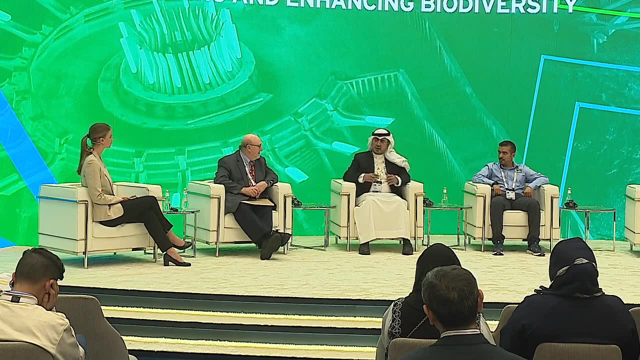 On the one side, you can reduce Or minimize the negative impact that you have, but on the other side- I know we've been talking about some tree planting initiatives, for example. Yeah, If you allow me, I would like to really first to comment on a very important point, that's with with my colleagues, what what mine company could produce as a waste, or or or a. 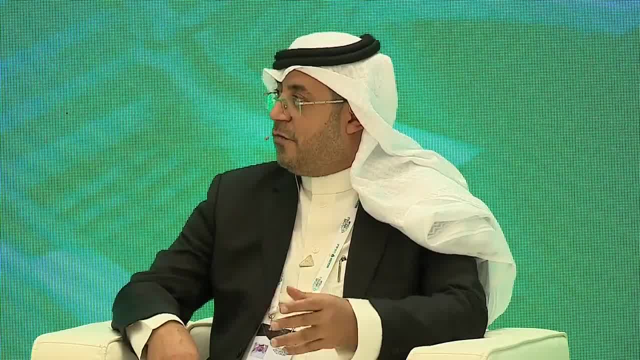 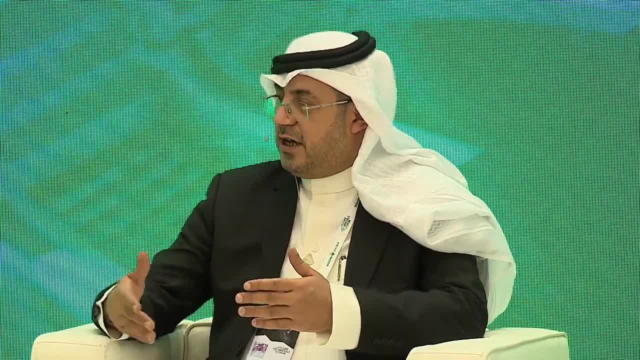 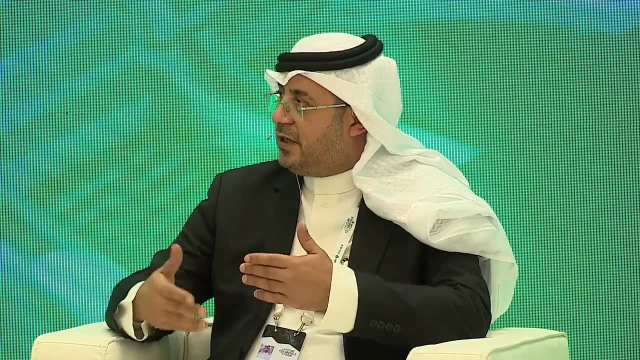 A secondary waste material that could be used in somehow with someone else, in utilizing that for, for, for, For Different way of production. And then the cooperation here between Us, I think is an example that we are not Only wasted, we are reusing the materials somehow in some way which is minimized the waste, and that that's definitely isn't encouraging, that the 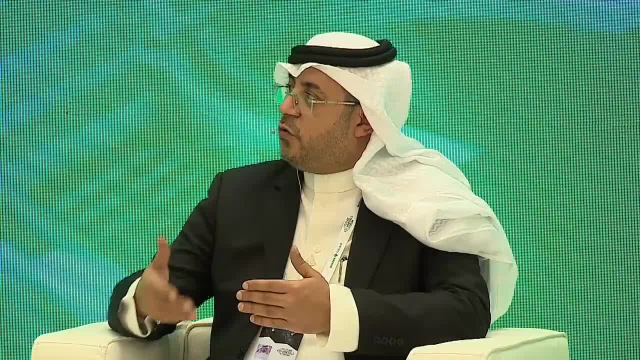 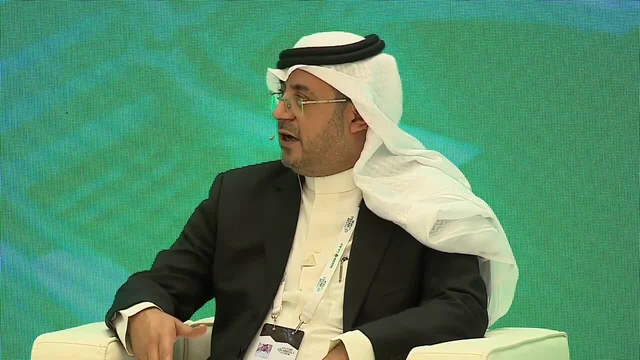 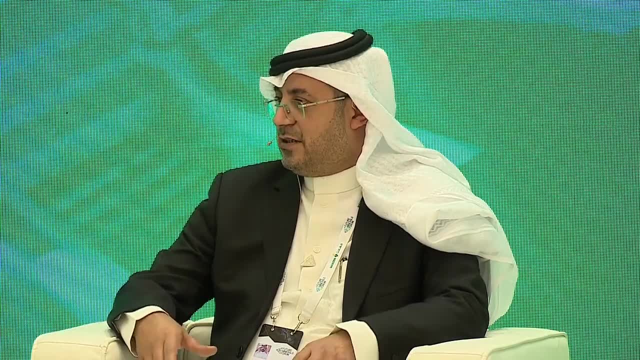 The company to look to the West as as how we can reuse it again and somehow or some way For the plantation that's modern, is committed now To plant up to twenty forty, more than Twenty million Plants, and an especially in such places like Saudi Arabia. this is very important initiative. it's not up to this. also, we are committed. 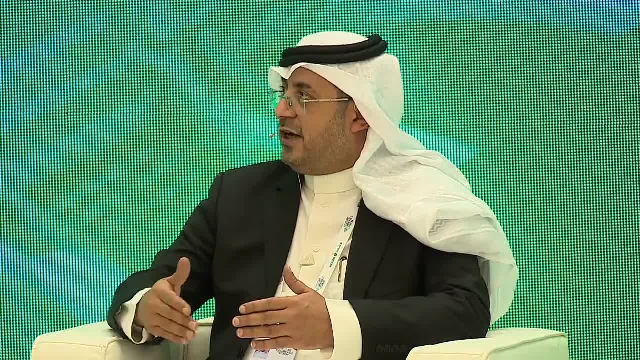 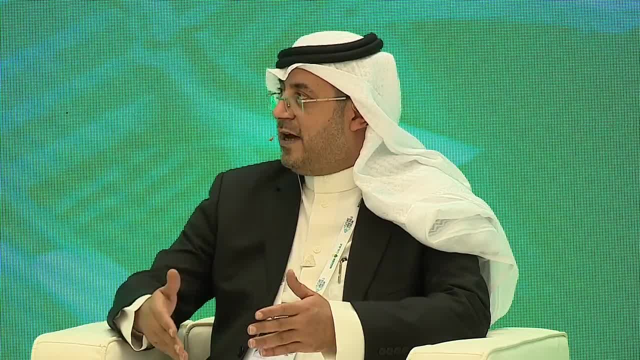 For the irrigation of this plant to be recycled water, so it's not only planting and using the main water, no, we are also committed to use Recycled water for this plant. and then it's scattered in so many places. in case a for for, really make that. 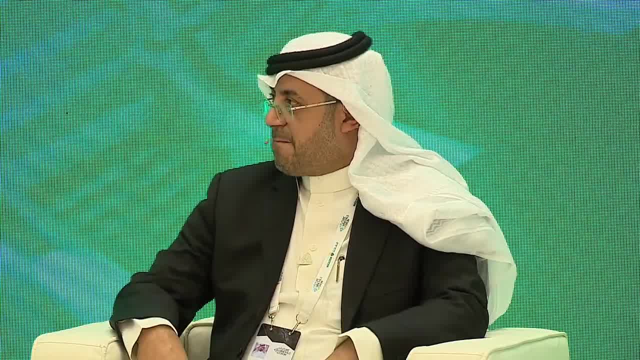 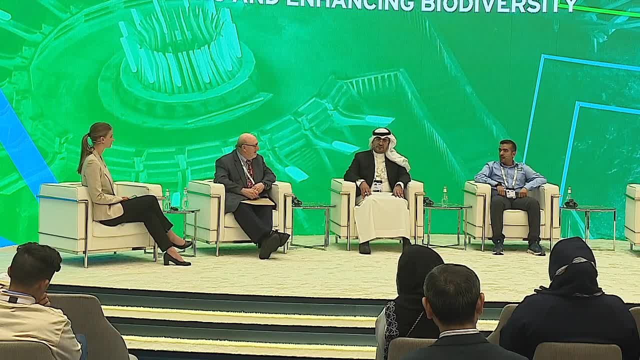 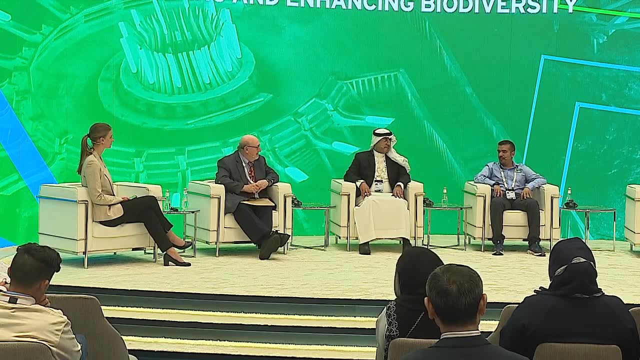 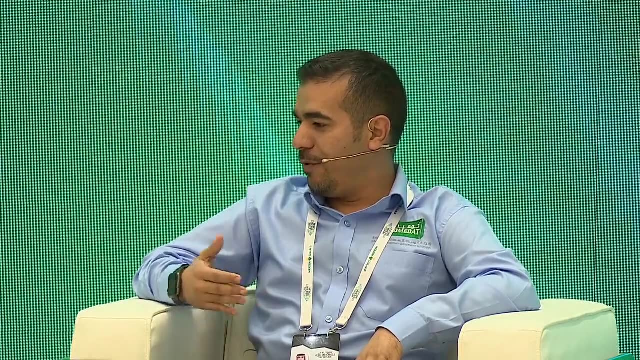 With what we call it a case a. so green, Saudi Great. I've seen any thoughts from you on how to enhance biodiversity, Actually, in To control the and help the people by the first city in the mining. I have more concentrate in the local community actually, because I, we believe that. 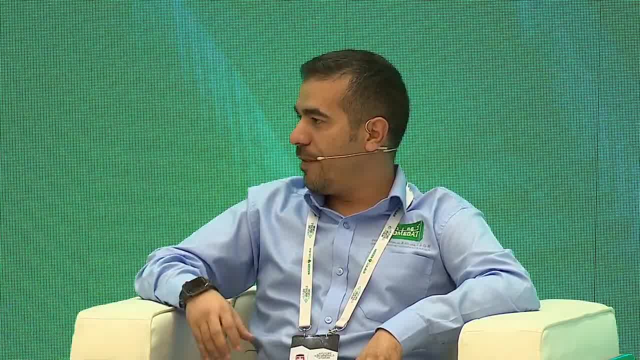 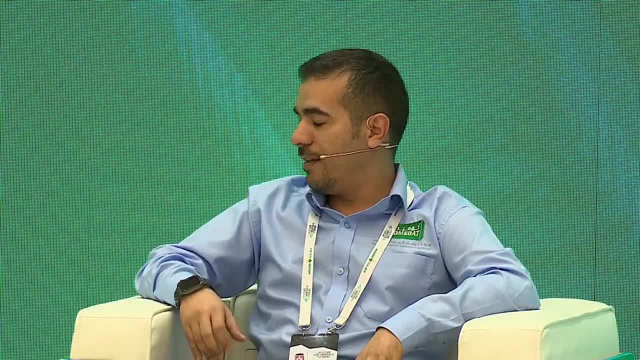 As long as you make the local community happy from the mining industry, he will support you and he will be, Be, Be, Be, Be, Be, Be And he will succeed as you succeed. also, and and the Mining goes, one of the biggest challenge in the mining- 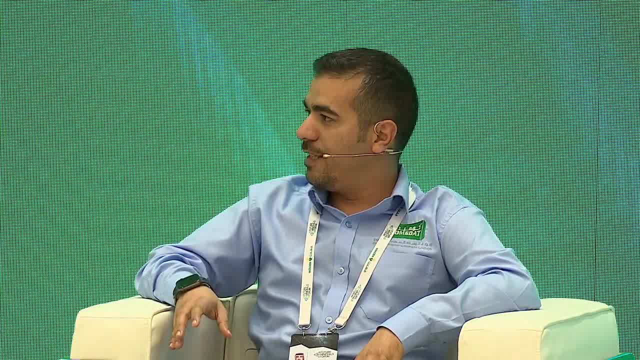 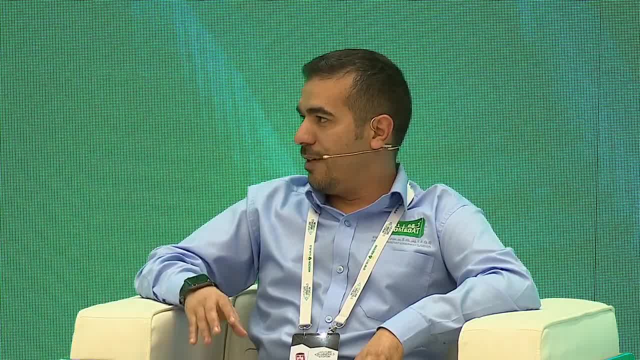 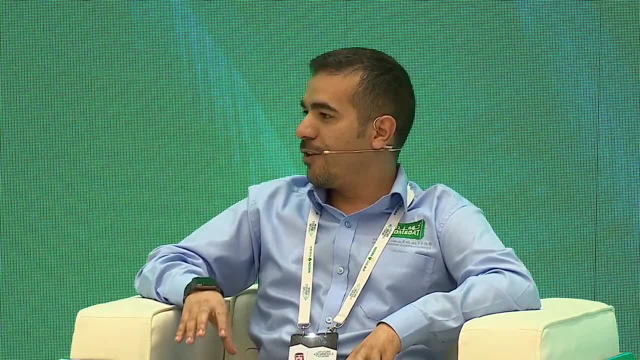 If you are not only in Saudi Arabia. Everywhere it is the local community. If local community help you to succeed, then you will be Succeed. also, if he's Don't like the mining at all, then you'll fail- definitely So local community it is. 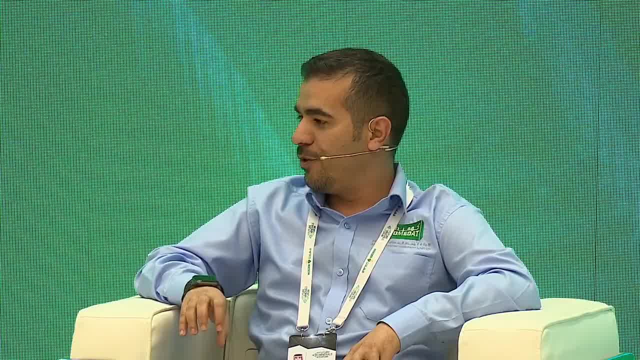 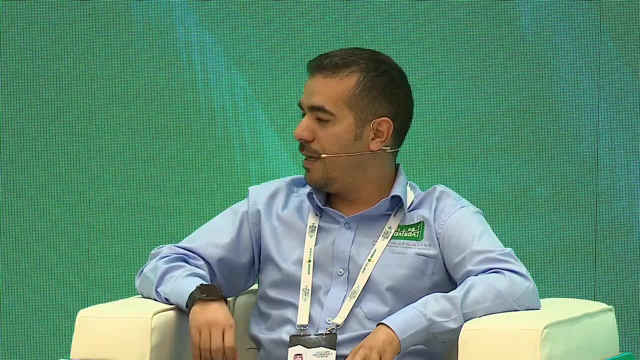 The main core of the business for the mining. He needs to involve him in the mining and he needs to give him part of the mining operation to make him happy and to help him as well as helping the company. So we've heard from two. 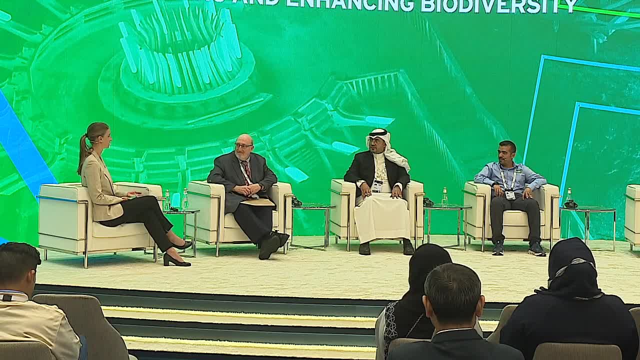 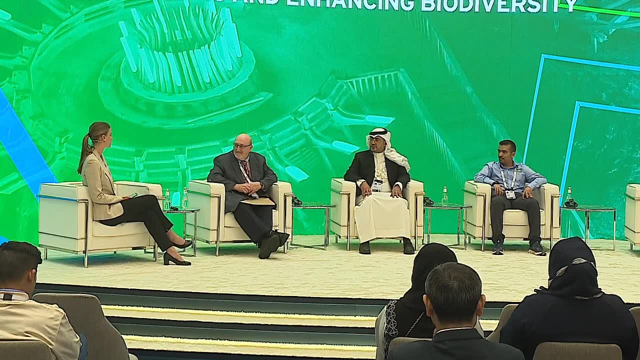 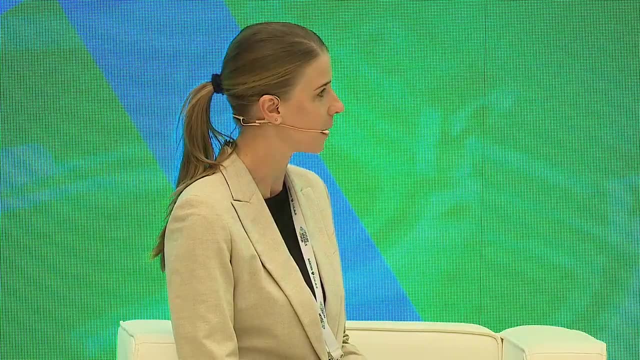 companies now, whose ESG policies have been built into the backbone of the company. but, Murray, speaking outside of the KSA, do you think governments should be more involved or is it really the companies themselves that should? No, it's a partnership, It always is. 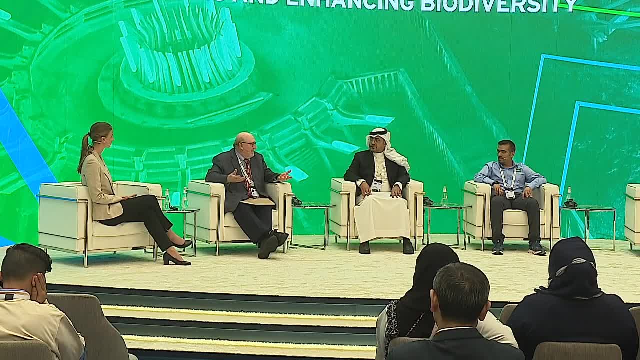 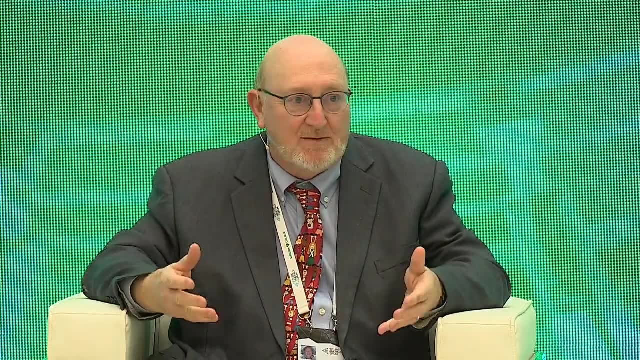 So our industry is always going to be regulated. We expect that. So they have to work in partnership, and I think that's something that we can see from this meeting. what the kingdom is really trying to do is actually bring government regulation together with industry and then, importantly- 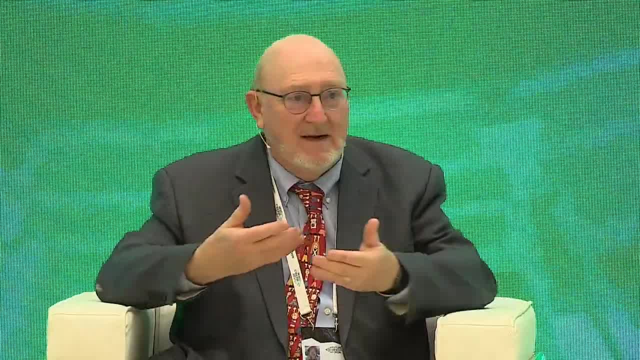 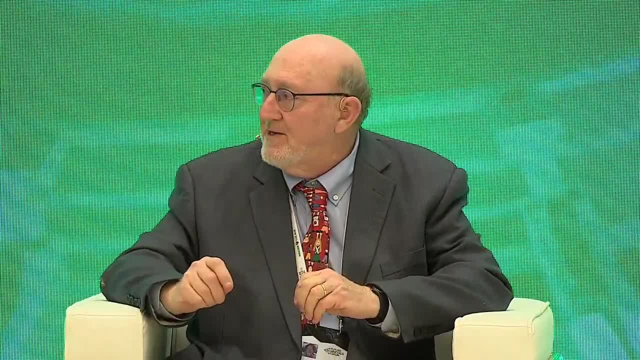 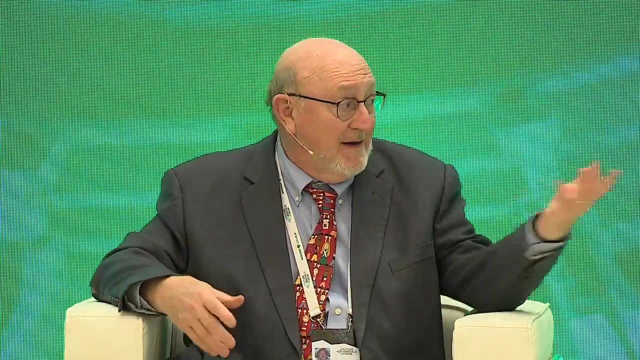 with the local communities as well. Another aspect: right, And the three work together to understand how do we make this work best so that everyone wins and there's essentially no losers. right, Including the biodiversity of the environment, But that's important because only if the community is. 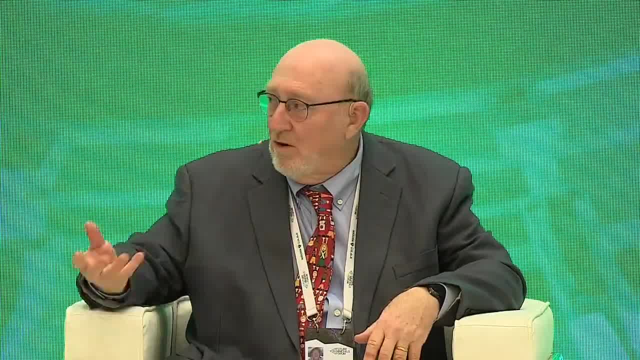 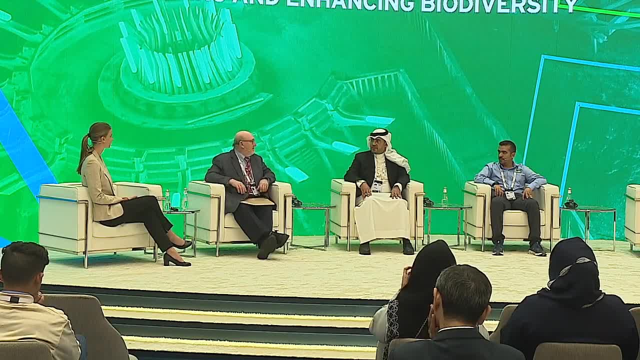 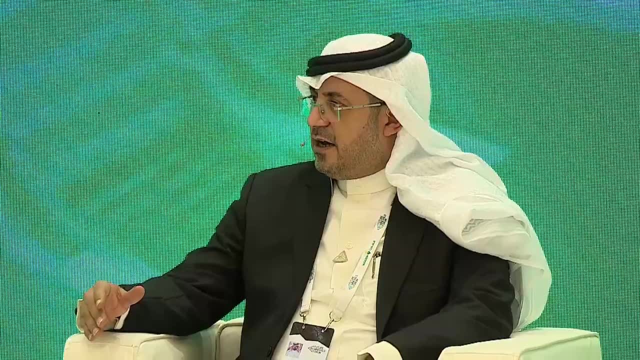 engaged, bought in and happy will we be able to do that? preservation, Sure, And any final thoughts for the audience, Some actionable takeaways, I think. referring to your question, your comments, I think, yes, the regulatory is important really to put the right regulation and ensure. 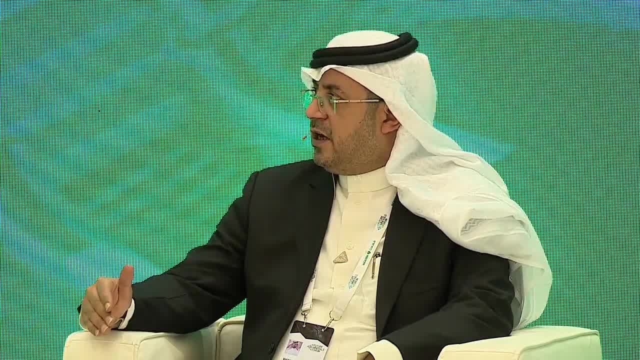 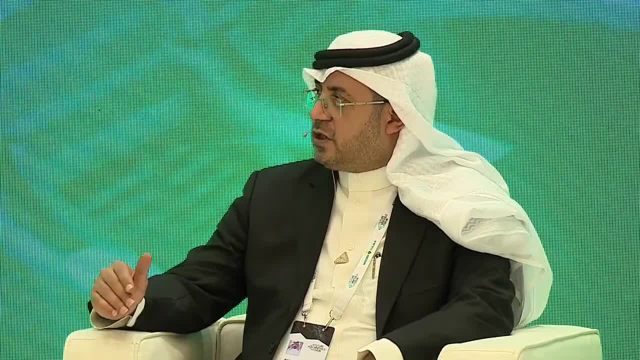 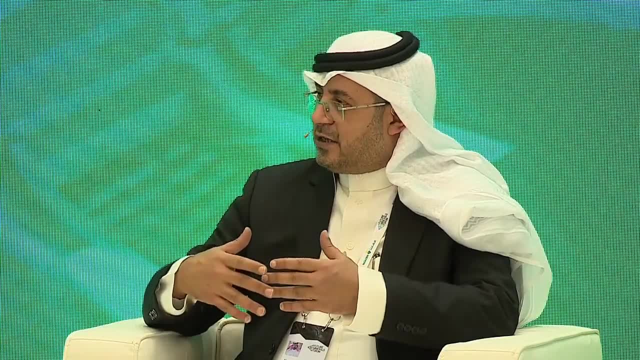 that all the mining companies are taking the responsibility for the biodiversity to the community. But what's also most important is to ensure that it is part of their DNA, because you don't want to be in a police situation. You need to be in a situation. 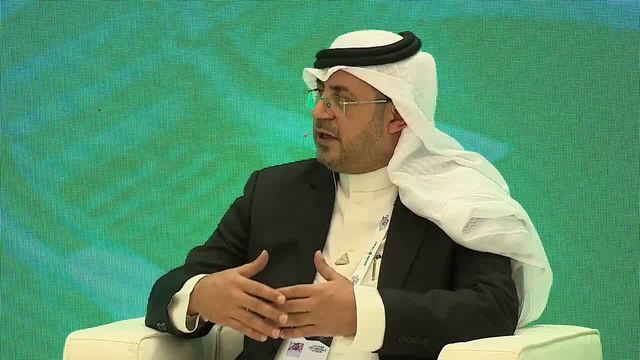 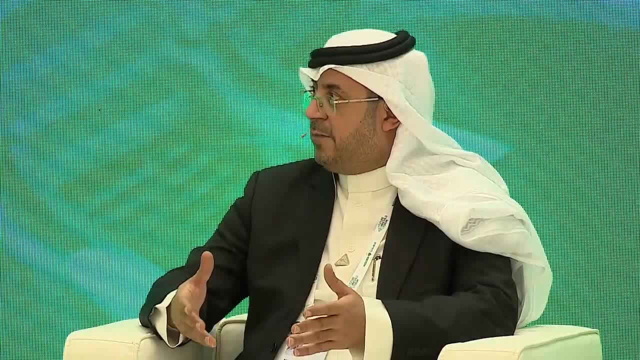 where the companies really hold the responsibility and be responsible for the mining company not to be in a police situation, And that's not only to the community, toward the whole country, toward the nation that they are working in. Because whatever that we do today, 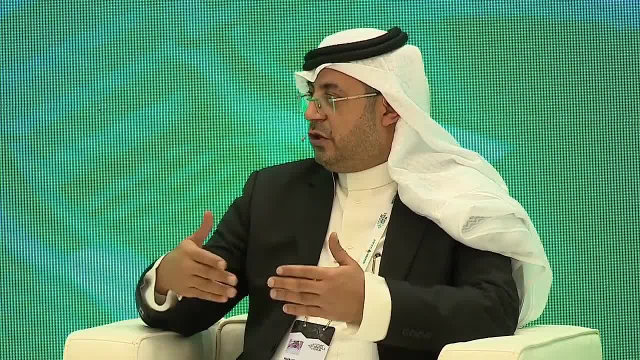 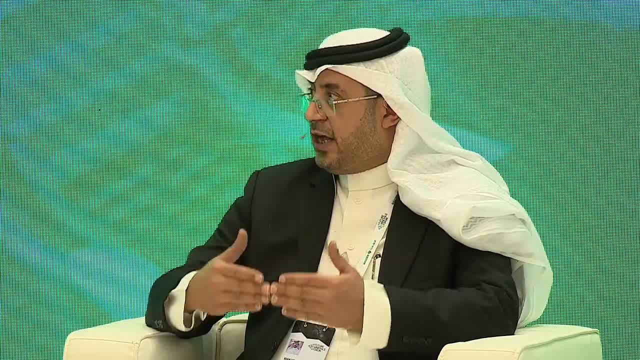 that will be for the future. So we need to make sure that, yes, the government, they do have the right policies, the right procedures, the right regulation, but, on the other hand, we need to work with the company, hand to hand, to ensure that. 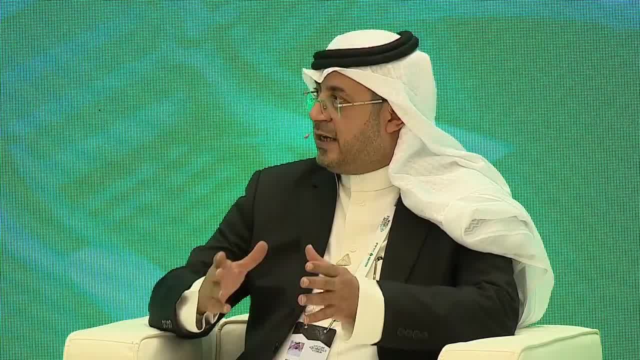 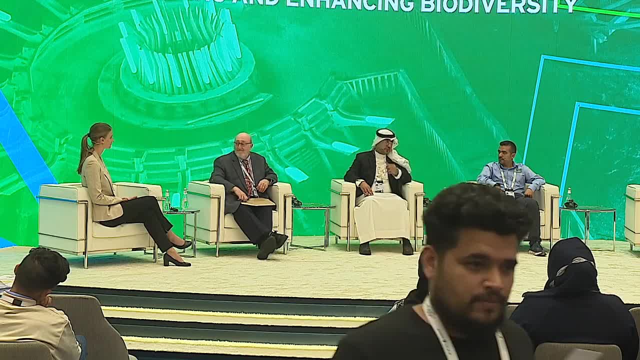 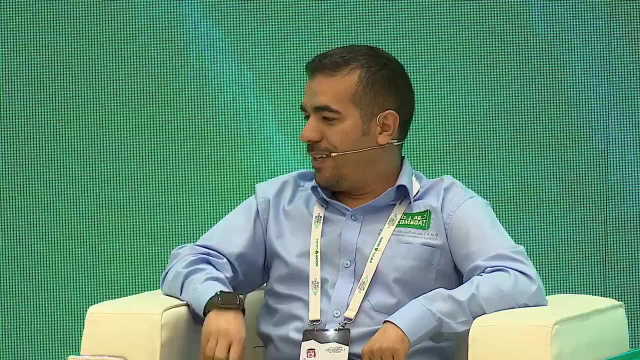 this policy's procedure is part of their DNA, And then they spread that to the other, and so on. Hassan, any final thoughts from your side? Again, Any final thoughts from your side. It is the final thing I want to say. It is: 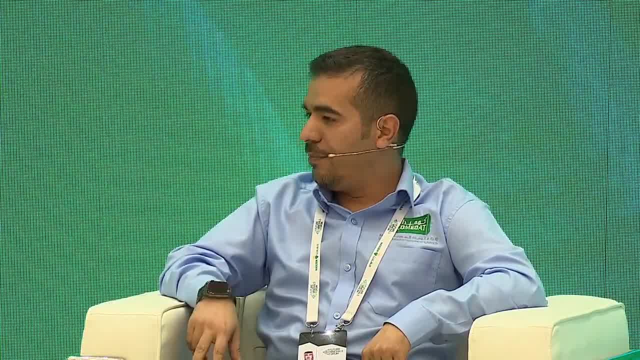 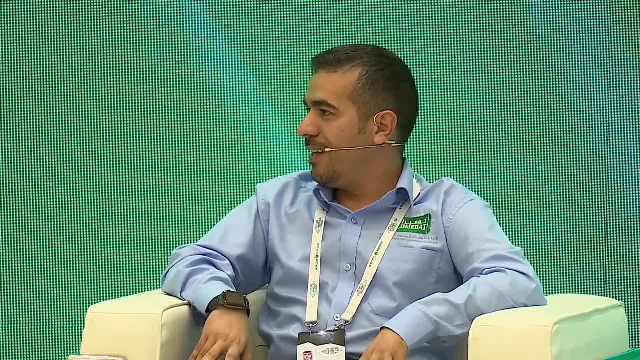 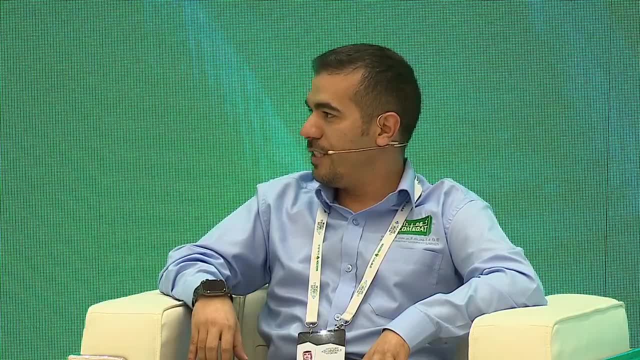 involve the local community, help the environmental, The mining. it does not mean it is something coming to destroy the earth. It is also to help to generate new things for the new generation. Without mining, we will not have the green energy Without mining.